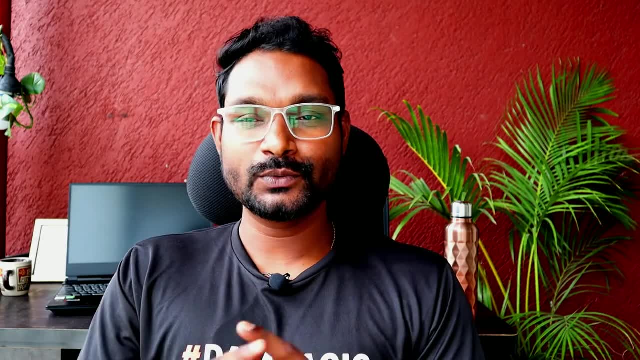 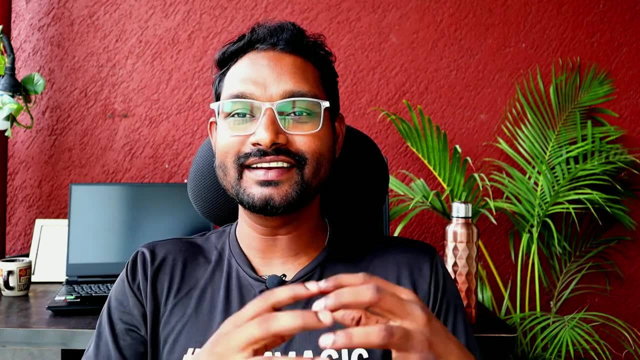 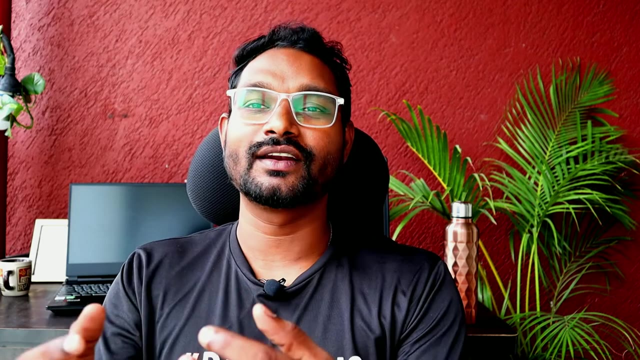 available on the internet. so the technique which used to collect or scrap data set from the different website available on the internet internet to our system and create a data set that we call it like a web scrapping, because we are going to the web and we are just trying to scrap the data and we are 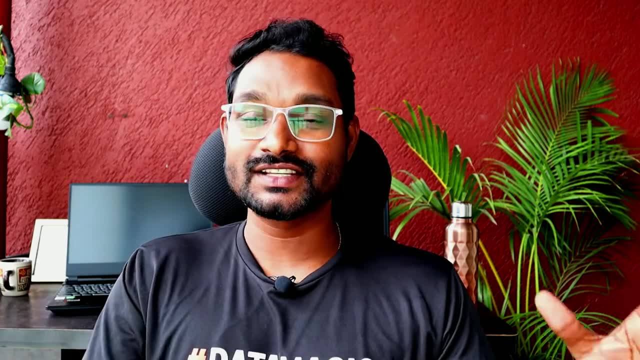 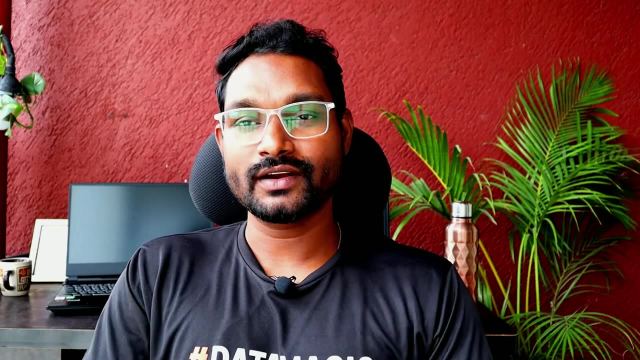 creating the data set by doing the web scrapping. now let's try to see a couple of examples where we need a web scrapping technique to collect the data set. for example, you want to analyze, like what kind of jobs are available in a market on the different site, because there are different job. 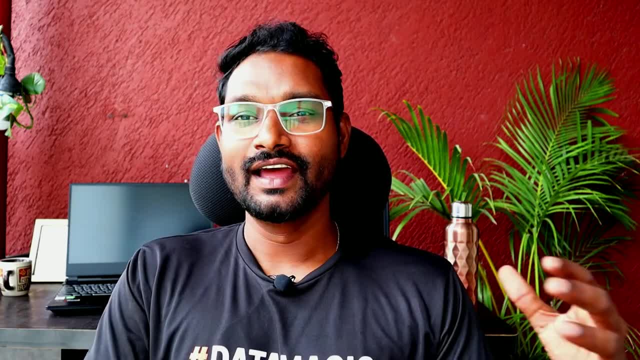 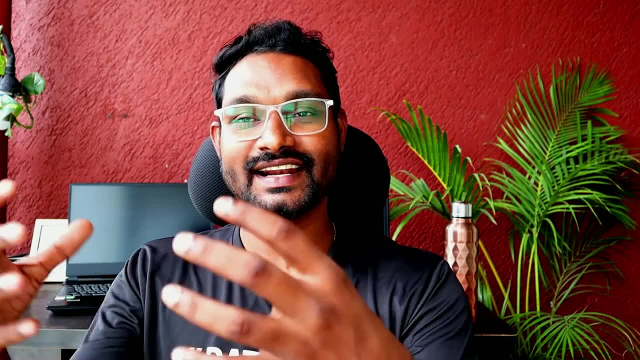 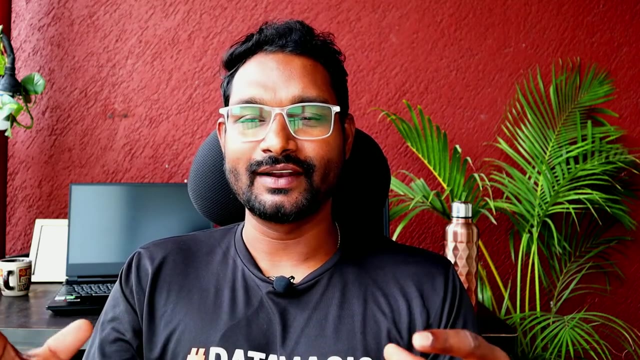 sites like there is a nokri linkedin, indian shine and there are so many like a glass door and so on, so you can go to these sites and collect the data set of, or the scrap the data of the different jobs, company names, what is the positioning, salary offerings, notice period and 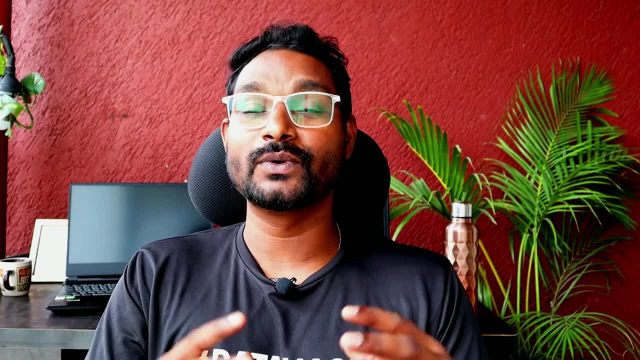 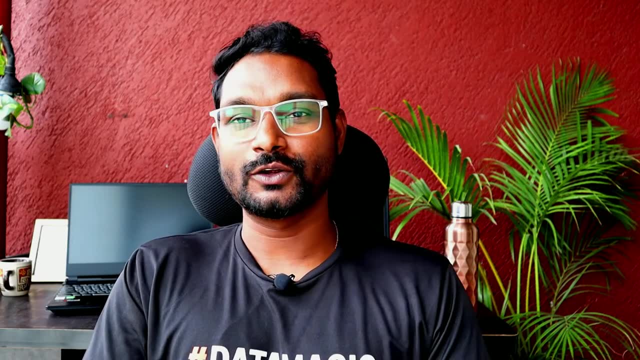 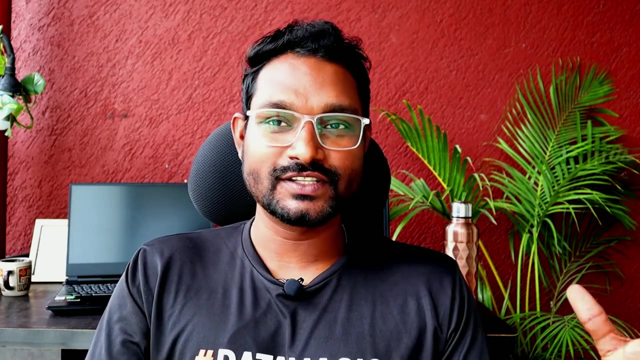 whatever details available on that site and we can collect it and create one data set related to the job. after that we can do the further analysis, like what are all jobs in a demand, what are all jobs paying high salary, or what kind of skills required, and so on. there could be other scenarios i could. 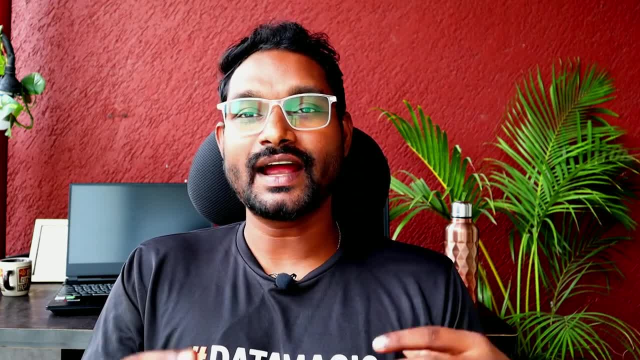 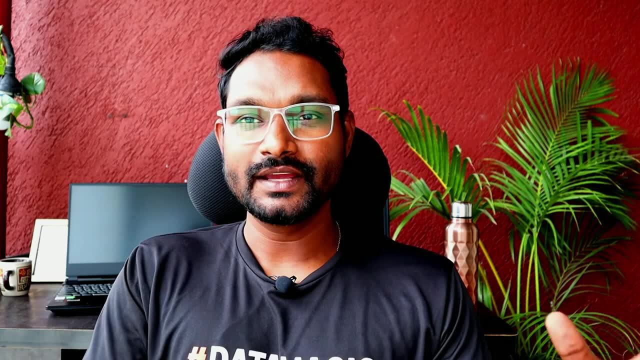 start using a web scrapping technique to get the data set that we need from the different sites- and there are a lot of startups are very well working in this area- like they are just scrapping the data set from the different e-commerce sites, for example. there is kind of a 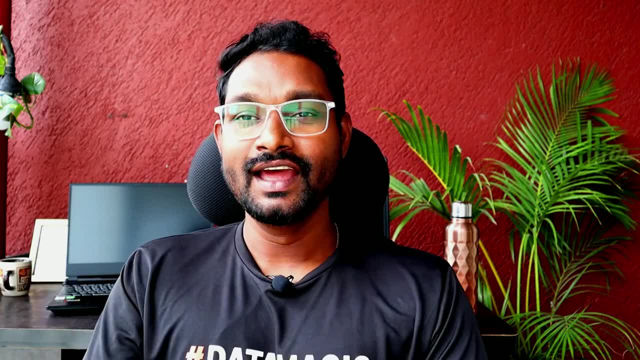 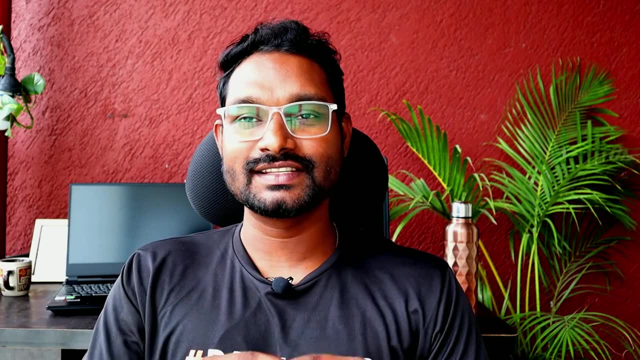 flipkart, amazon, ebay and there are so many big e-commerce sites, so these startups are going to this e-commerce site collecting the all the data from their site- different product price- and they help to the other e-commerce sites like, let's consider, they will scrap data from a flipkart and 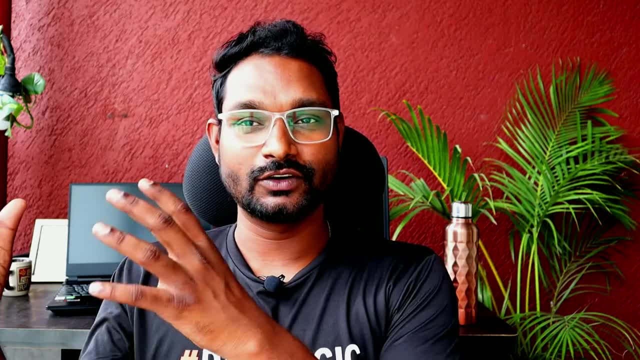 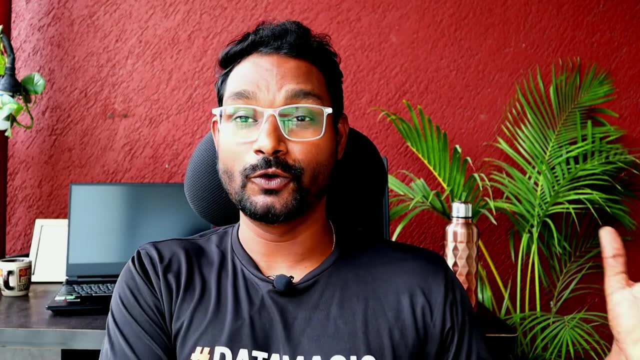 they will say like: these are the products listed on your site and these are the product listed on the ebay and flipkart. compared to whatever the pricing available on the ebay and flipkart, your pricing is high or low. let's consider if amazon interested, they will buy this data and they will. 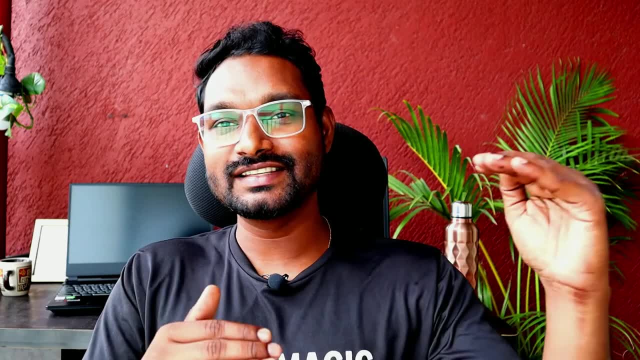 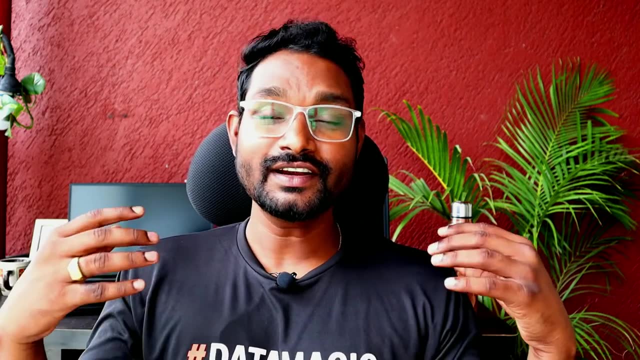 see, like, where are the areas where they can reduce price or increase the price of their product based on what is the competitive market is okay, so this is just a couple of ideas. so there are different business problems that can be solved by scrapping the data which is publicly available. 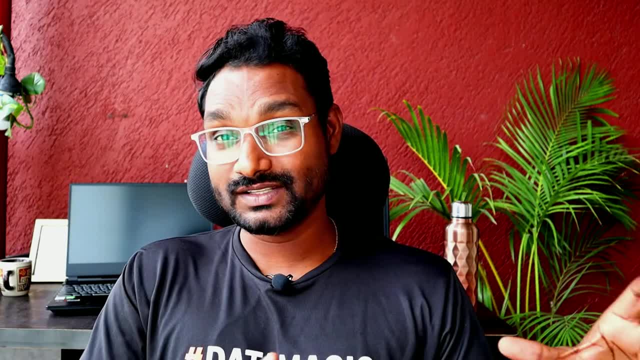 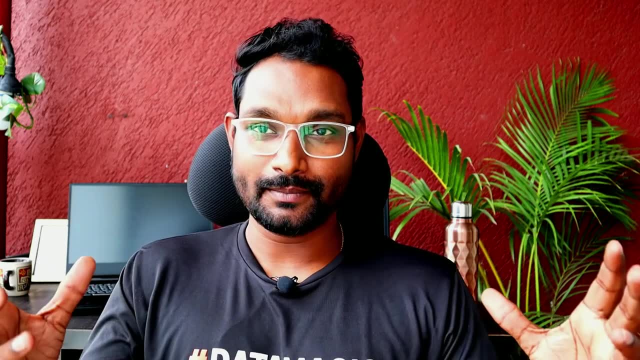 on the websites. okay, so that's all. hope you've got idea about like, what is web scrapping and where exactly it can be used. okay, so now let's go to the computer screen and see, like how we can do the web scrapping. okay, so before that there are the two kind of websites. okay, so one website could. 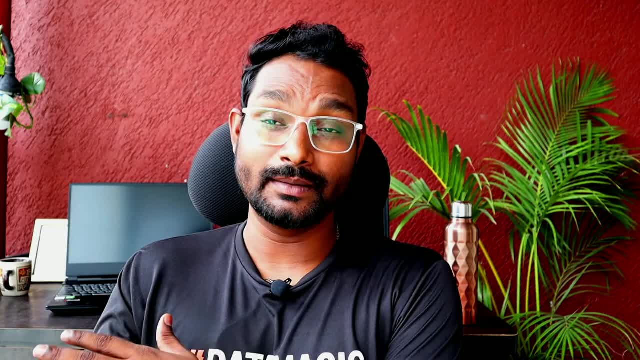 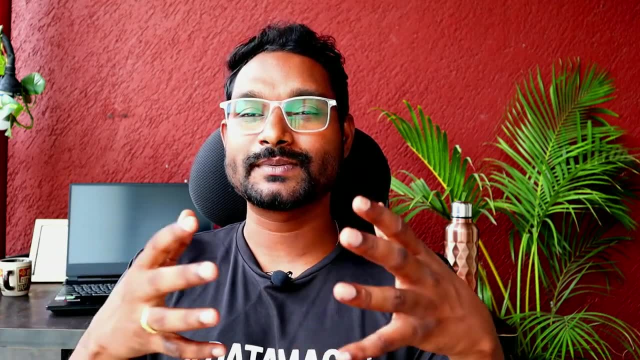 be like a static kind of website and another type of website that could be the dynamic static websites of the website. its whole content is static, so once you make a request to that website you can get all the website content in the response. but dynamic websites are the. 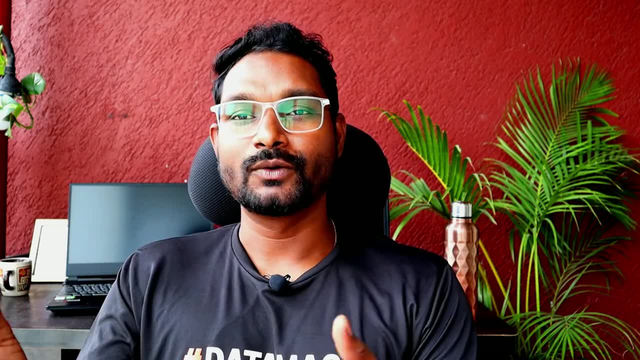 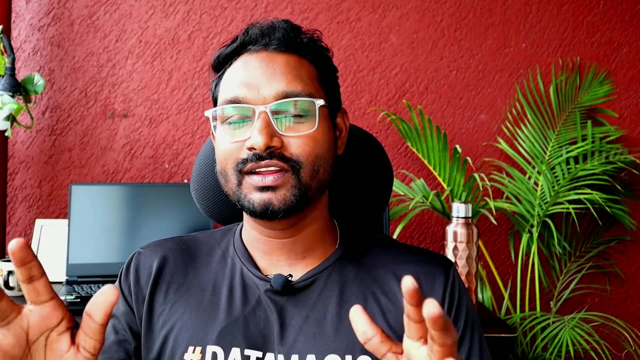 website where you will just get access to the one page data and once you perform some action, then the other data will appear on that website, so that we call it like a dynamic website. okay, don't get confused. as of now, we are just going to focus on the static part of the website. okay, so we are just 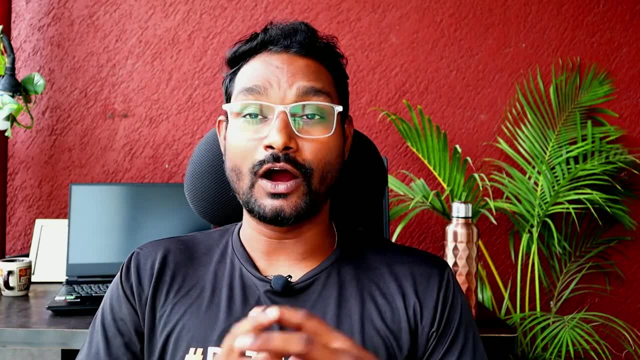 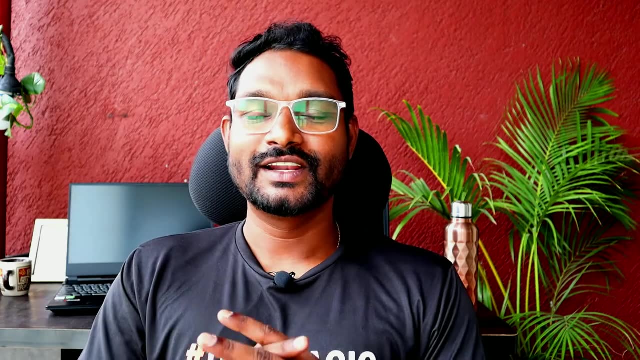 going to deal with a one page. so i'm going to show the practical, like how we can make use of a beautiful soap library, which is available in a python, to scrap a data set from the different website. so let's go to the computer screen and start doing the web scrapping. so just before 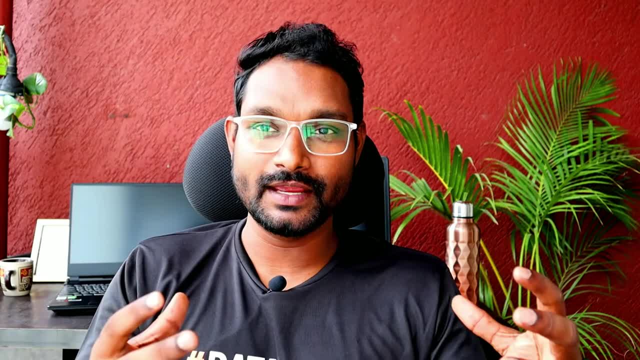 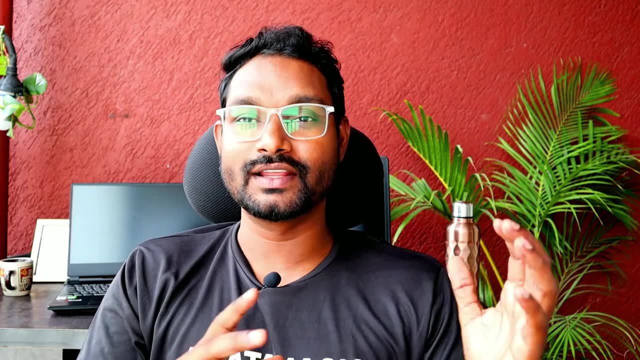 if you want to know like how to do the web crawling with the help of a selenium api, then please let me know into the comment box. if i found that more comments and more people are interested in doing the web crawling with the help of a selenium, then i'll try to create a new episode on how to do the. 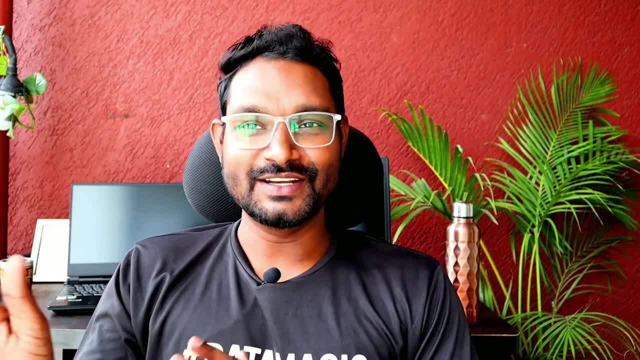 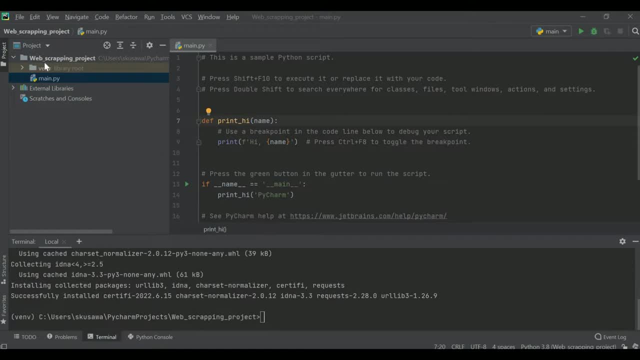 web crawling with the help of a selenium. okay, so now let's continue. now you can see my laptop screen and on my laptop i have opened the pycham id. inside of that, i have created one new empty project with name like a web scrapping project, and this is a completely empty project. whatever this sample. 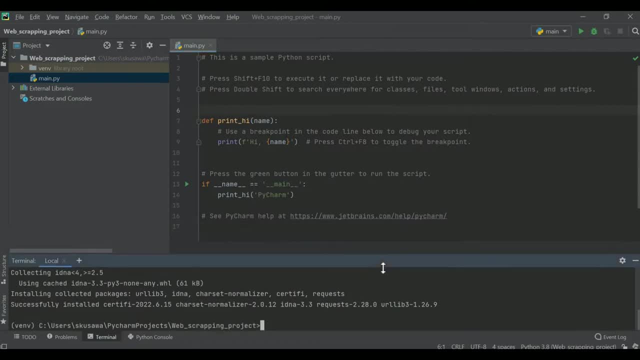 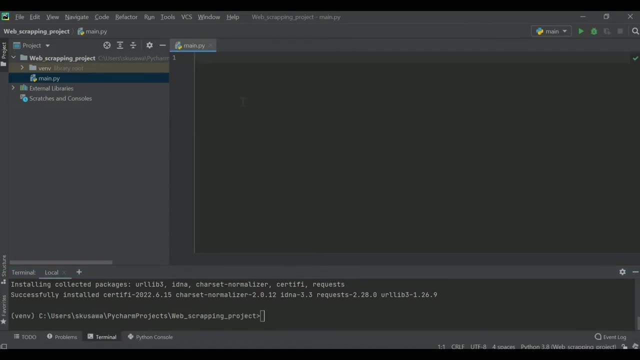 code. you can see. this is the by default provided by the pycham id whenever you create any new project. so we don't need this code. so let me just remove it and here we'll try to write our whole web scrapping code. so today we are going to scrap the code from the job portal. okay, so we have. 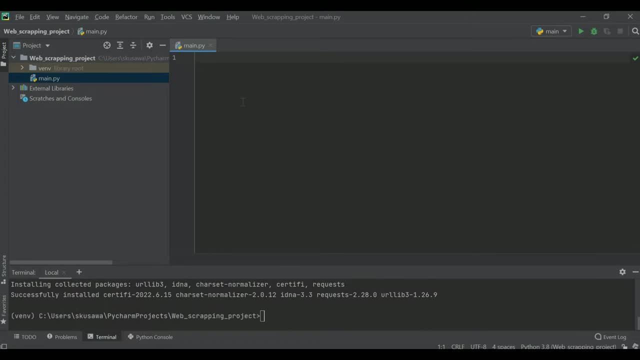 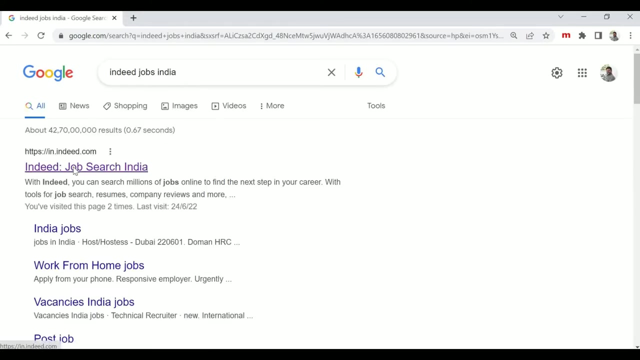 selected like an indeed job portal and from that we'll try to extract the job details. so let me just go to the browser and let me show you, like, what exactly page we are going to access and what kind of details we are going to fetch. let me just search for indeed jobs, india, and this is the first link. 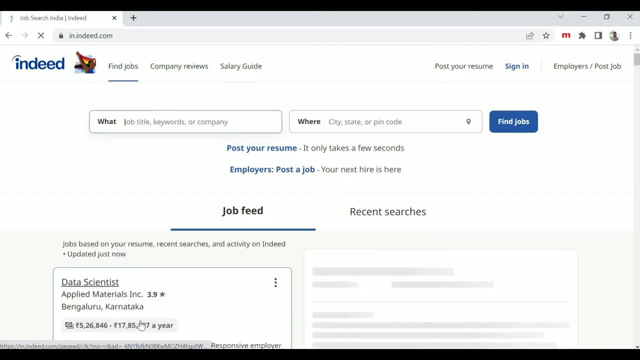 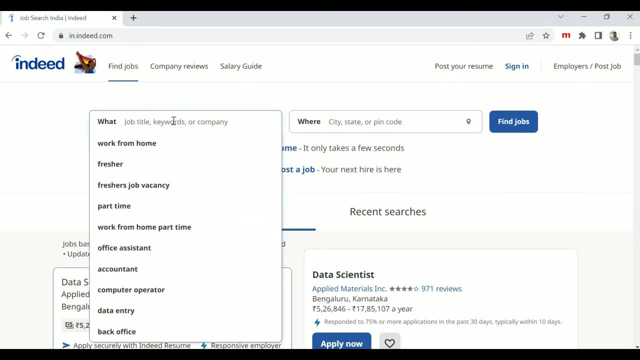 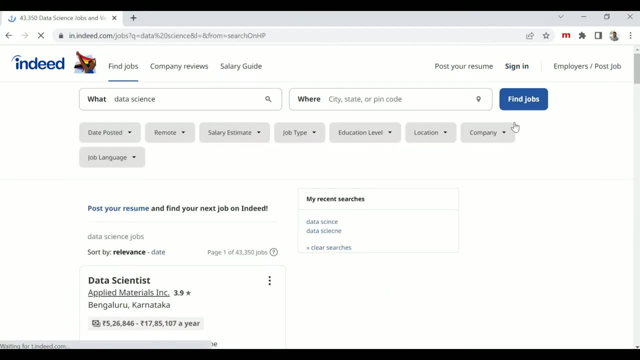 and on this link you can see that we have the listed jobs. so if you want to search for specific jobs, like a java related job or data science related job or any post, you can just put here the keyword like data science jobs, okay, and just find the jobs. so it will. 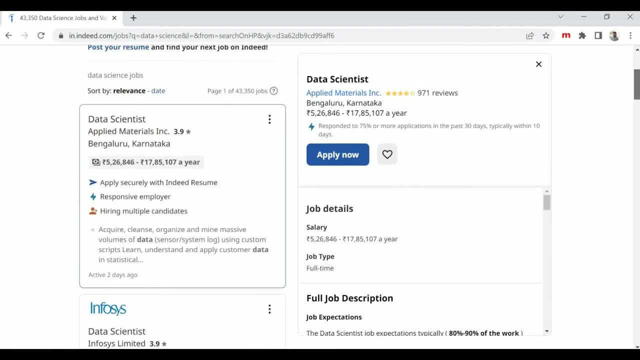 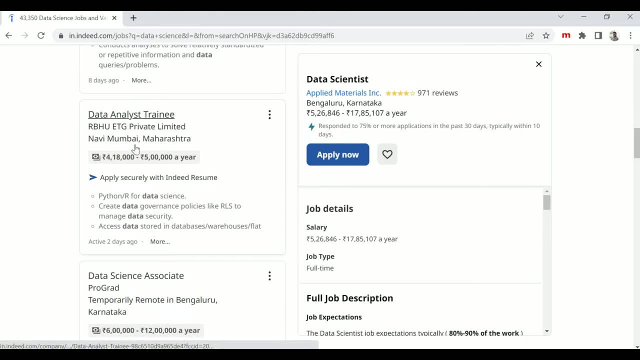 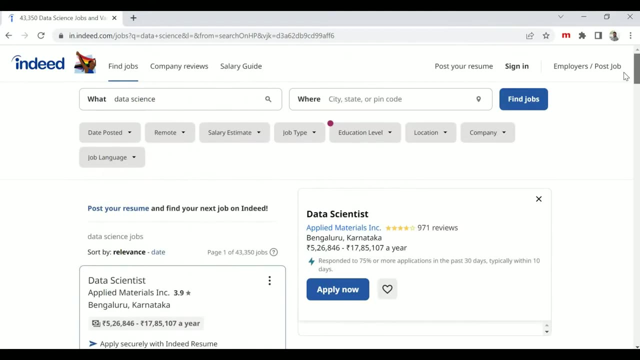 give you the all the jobs which are related to the data science. so you can see that i'm having a lot of jobs available over here related to data science. there is a job title, company name, location, ctc and other job details. so we are going to extract all these job details in our python program and we 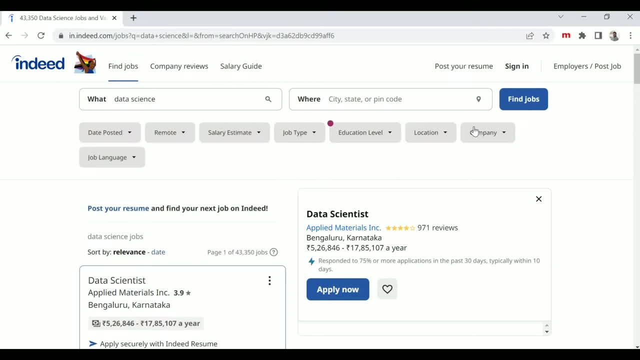 are going to form one kind of a data set, so let me just try to take this url and let me go to the code, because we are going to access this url and from this url we are going to get the job details. whatever the page content we have, we are going to extract the each job details, okay, so let me just 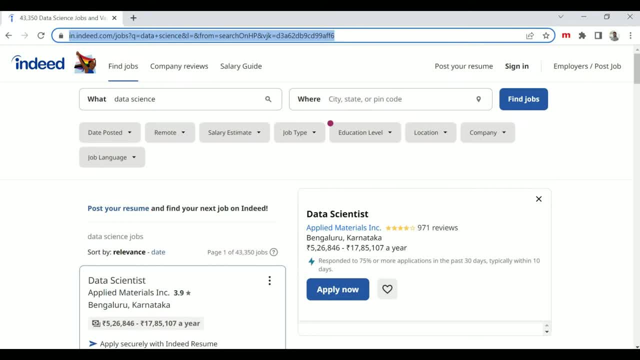 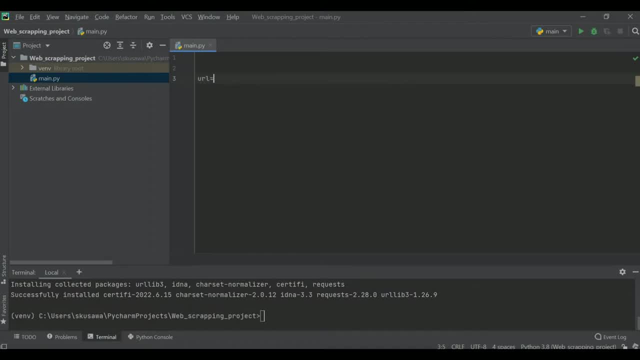 go to the code. let me just copy this url first, and now i'm navigating to our code, so let me just save this url in one variable so we can later use it. okay, so that's it. so this is the page from which we are going to fetch all the job details, or we are going to perform the web scrapping. 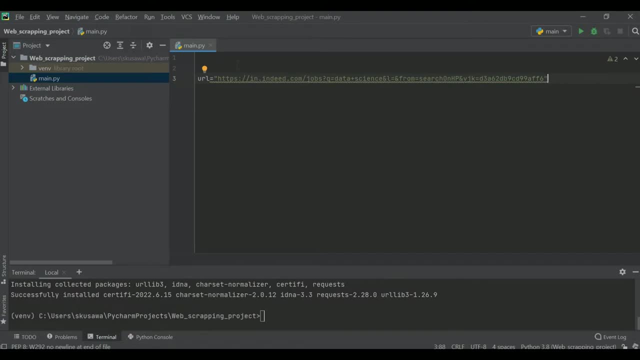 so for this web scrapping we'll be needing the two libraries. okay, so first one is like a request. this is the api which will help us to fetch data from the internet, from the url, and once we get the response or data we need- like a beautiful soap is a one. 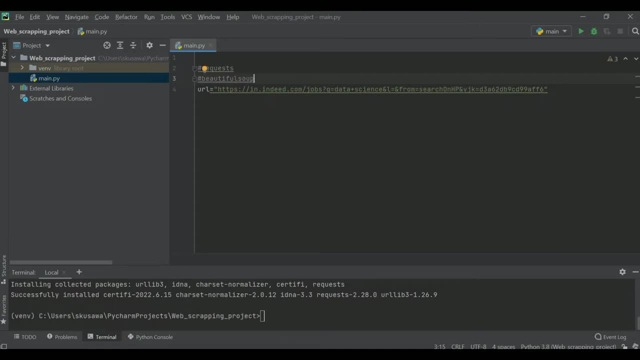 another api or library we could say which will help us to parse this all response data and it will help us to find the data of our interest. for example, on site we just want to find, like what is the job title or what is the company name, so we will be able to fetch. 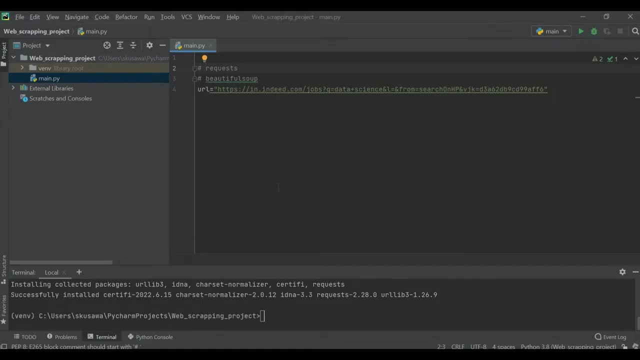 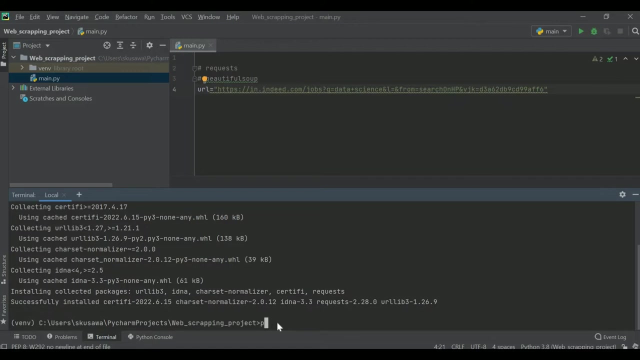 it. okay. so let's come back to our id and here you can see that let me just try to install these two libraries. so i'm going to terminal. okay, so here you can see terminal and on there we have to type a command to install the request api. so i can type like a pip: install requests. it will install this. 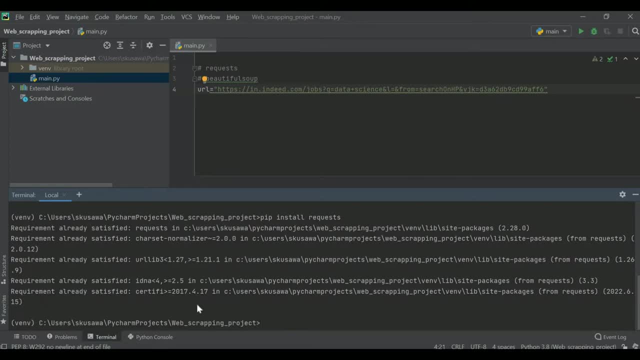 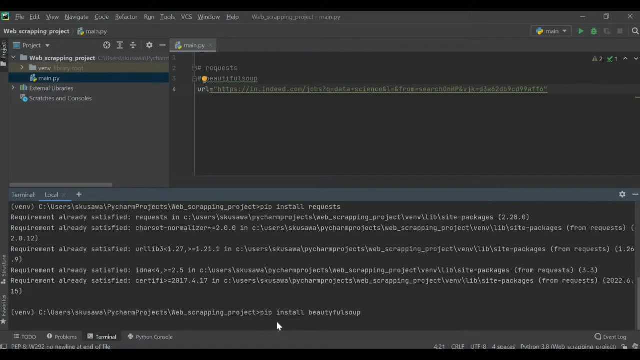 request: api: okay, so you can see that i have already installed. so it is saying like: requirement: satisfy it. now i'm going to install the beautiful soap. so let me just type like a pip: install beautiful soap and let me just try to install. so i'm getting some error like: find version that satisfied okay. 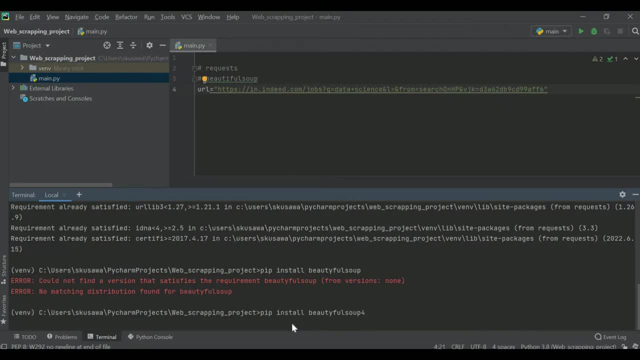 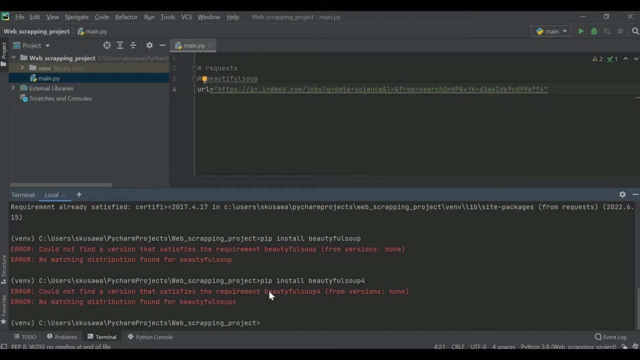 so we have to use a command like beautiful soap. okay, pip, install beautiful soap. so it will install this beautiful soap library. okay, so i'm getting error. it is saying like distribution is not matching, so whatever i'm typing over here, okay, so this beautiful soap. so there is some mistake in this. so if you don't know anything like what exactly the 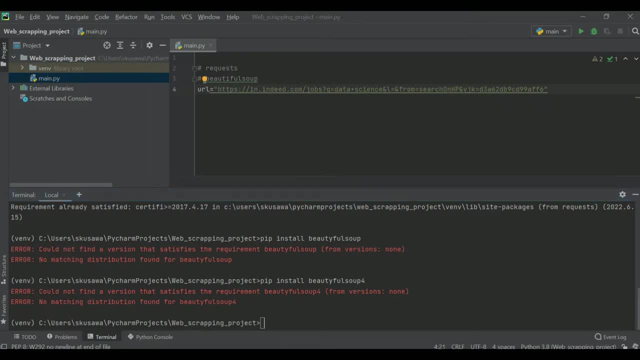 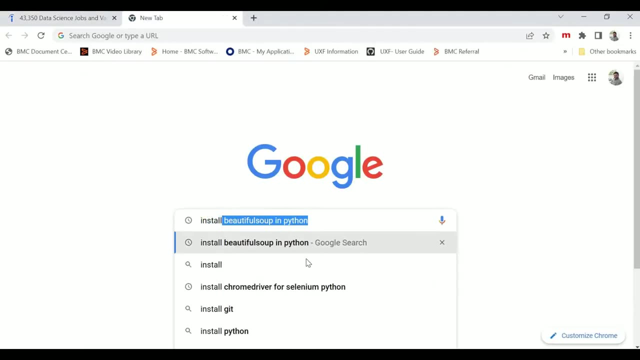 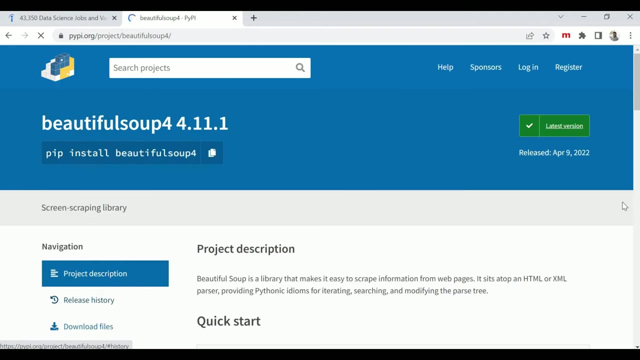 installation command. then you can just go simply to the google or the browser and just open a new tab on google and search like: install beautiful soap in python, okay, and you have to visit this pi pi dot org site. so once you visit this site you can see like this is the command: pip install. 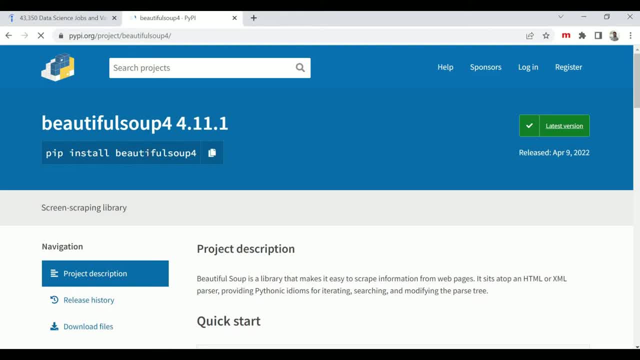 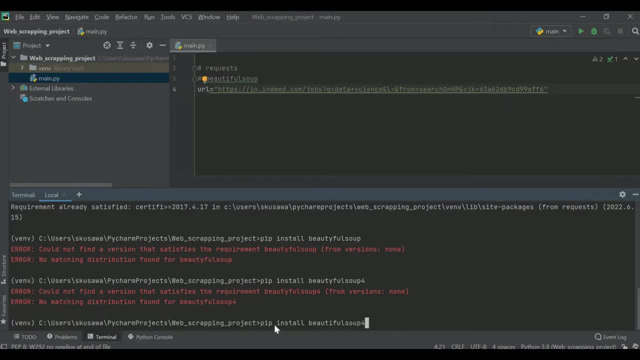 beautiful soap. okay, so you can see that i was making mistake, like i was using y instead of the i, so let me just copy this command. let me just go back to our id and let's paste it and let's try to run it. okay, so here you can see that it is installing and 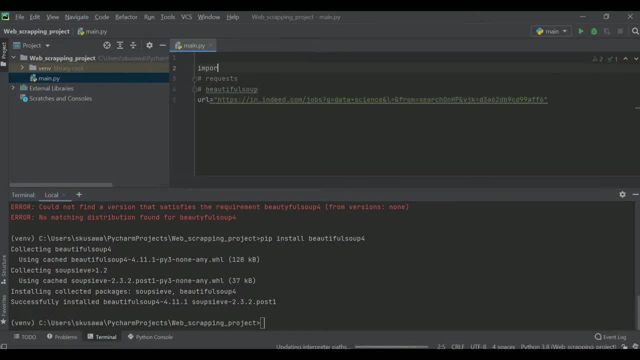 it's done. now we can import these libraries. okay, so let me just import requests. okay, so it looks fine. and now let me just from this beautiful soap- we call it like a bs4 module, and from that i am going to import this beautiful soap. okay, now we have imported, so let me just 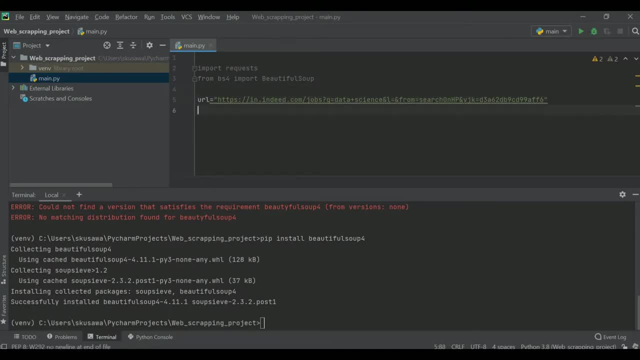 these comments. we have imported these, both libraries. Now let me just try to access this URL content. So for that we have to make use of a request And it has like a get method: okay, request dot get, And inside of that you have to pass the URL. So this is the URL from which we. 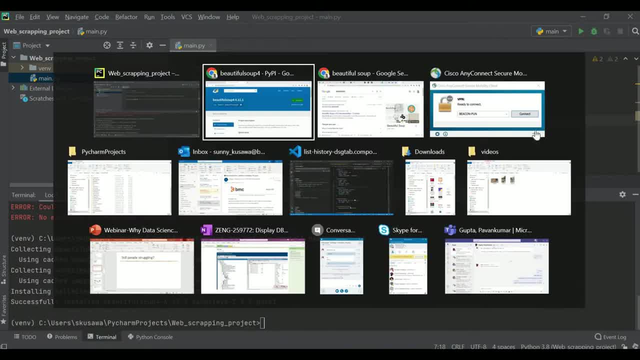 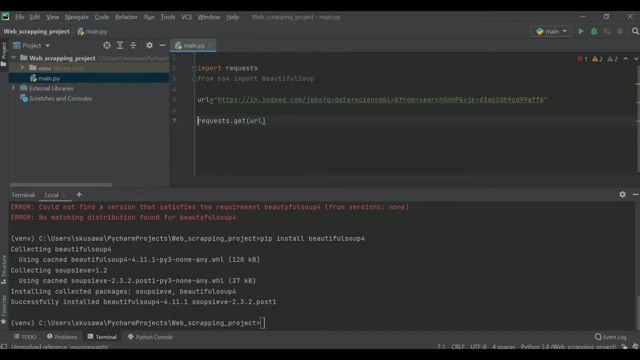 want to fetch all the data. So this is the same URL which I have just shown you over here. Okay, so this one is the URL. Let's come back over here. So on code, So whatever request we are sending, we'll get a response And that response will have the all the page content. So let me just 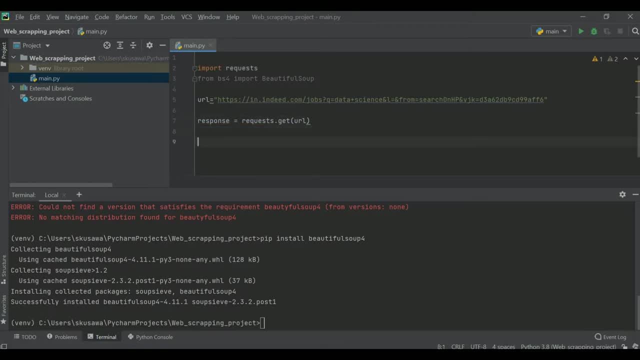 store this response in one variable and name it like a response. Okay, so this response will actually object, which will have the HTTP status code whether this request is success or not, And inside of this response we have the content. that will show the exact content. 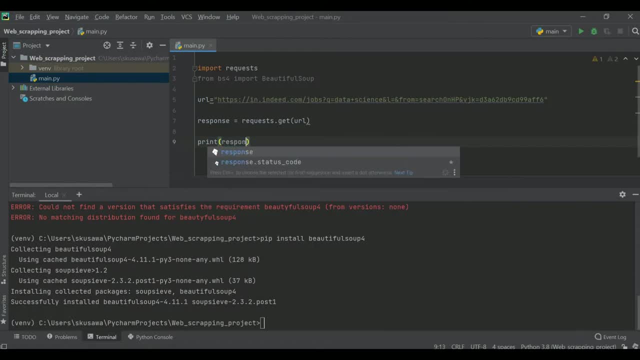 So let me just try to print that content. Okay. so response dot content: Okay, and that's it. So it will print the actual content And if you want to just see the status code, it will print the actual content. And if you want to just see the status code, 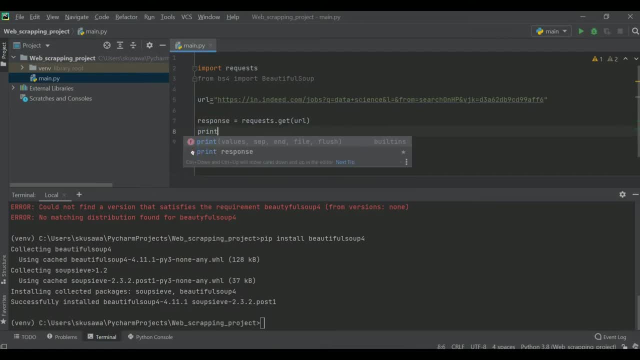 we can just print like a response. So let me just say like a print and response. So it will just print the like HTTP status code whether request was successful or not. So let's try to run and see like what happens. So let me just right click and click like a run main And let's 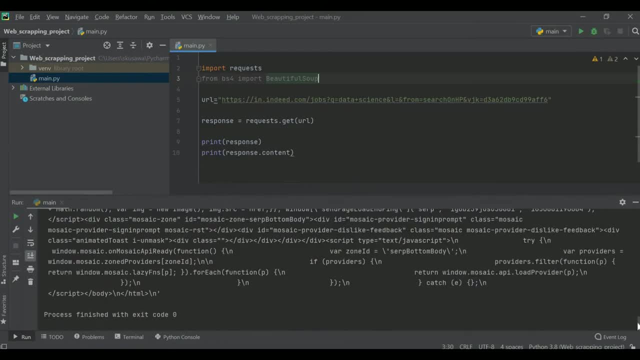 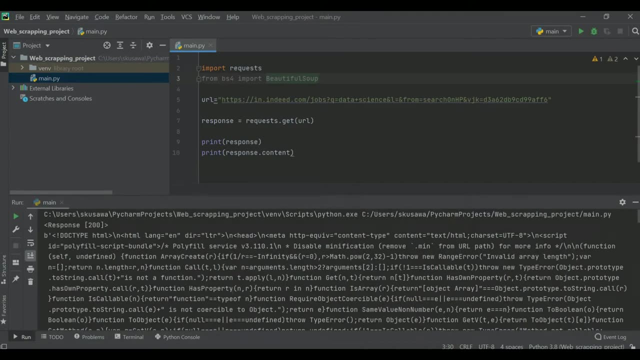 wait for the results. Okay, so you can see that we are getting a big, huge response, So you can see a lot of stuff we are getting. Okay, so this is the response from that URL. So once you hit this URL, these are all data we are getting And you can see this response: 200.. So, 200,. 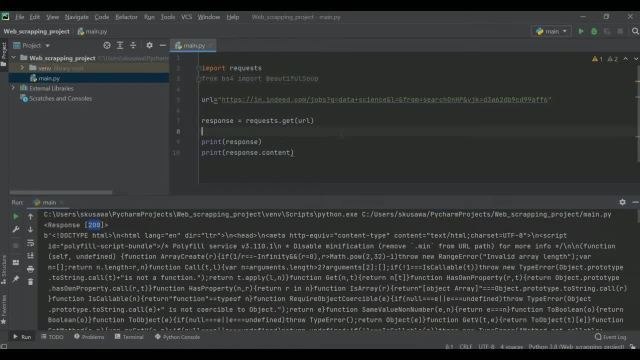 200 means like it is a HTTP. Okay, it means our request is working. fine. Now we got this data, But rather than this data, we are interested in the HTML content of that page. So whatever the HTML content available on the page, that is the more important. so we can extract the field. 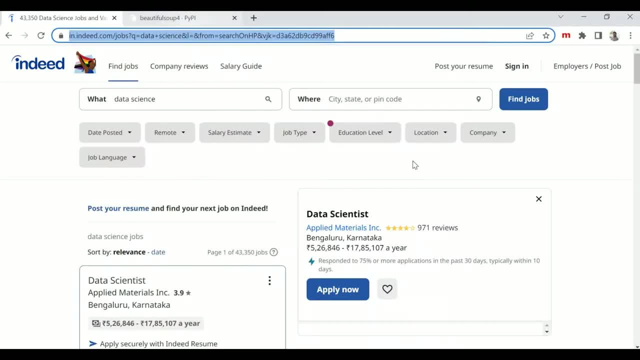 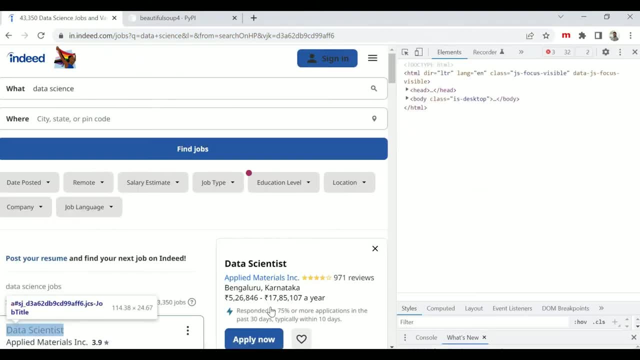 So what I'm talking about, let me just quickly show you. So let's go to this page And these are the different jobs. click on any job, right click and say like inspect. So once you say inspect, so you will get this developer to. 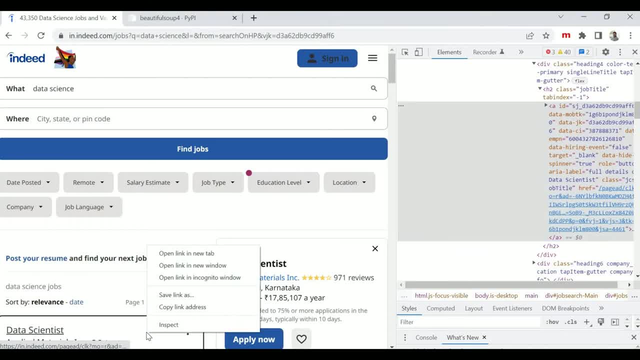 also Okay. so let me just repeat: you can go to the any web page, you can click right and click here inspect, And you will get this developer tools open And here you will find, like whatever item you select. So let's consider, if I just go here and select right, click and inspect, I was 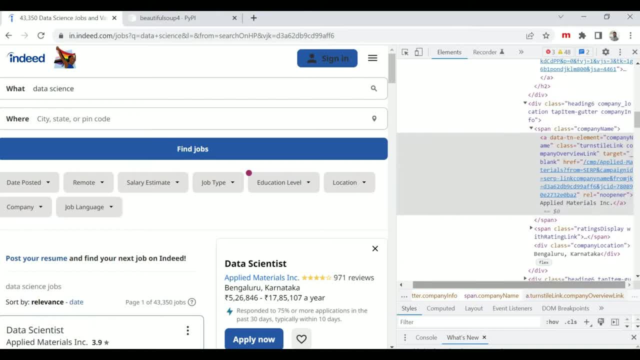 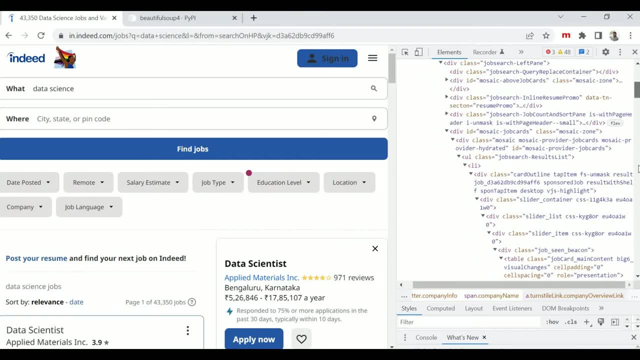 able to see related to that code. Okay, so you can see that this is applied materials INC. So I'm able to see like this: applied material INC. So this whole is a HTML code of this whole page. Okay, So as of now, we are getting very junk response. we just want to. 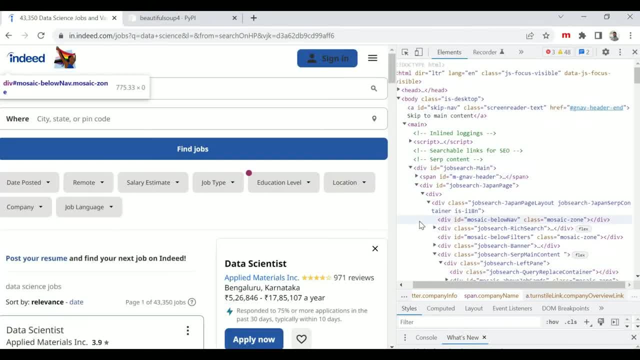 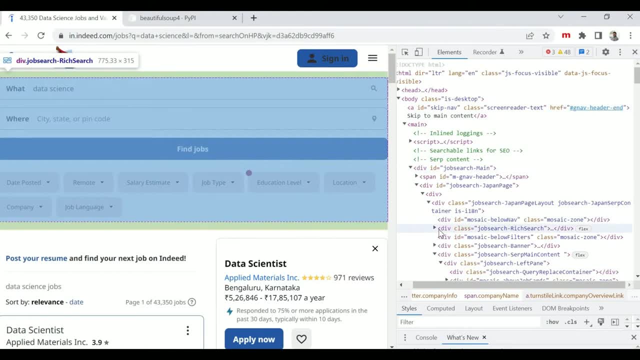 access this HTML part or HTML content from it. So how to access this whole HTML content? because once you get access to whole HTML content, then only we will be able to see: like okay, so this deal belongs to this highlighted portion. Okay, if I just scroll down so you can see that. 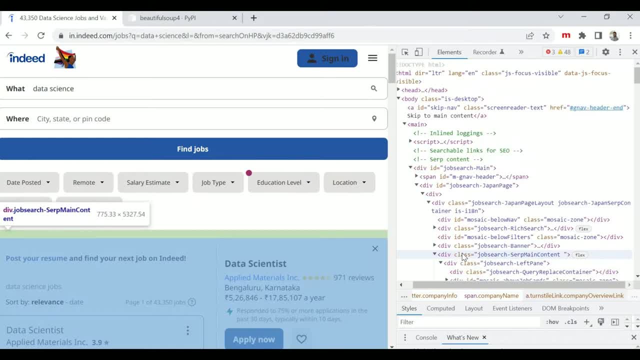 whenever I'm going to the next deal. so this is the highlighted left hand side part is related to that. if I go again deep so you can see that these are all the job list. Okay, if I just keep scrolling I'll be able to get go inside a more details. Okay, so you can see that. 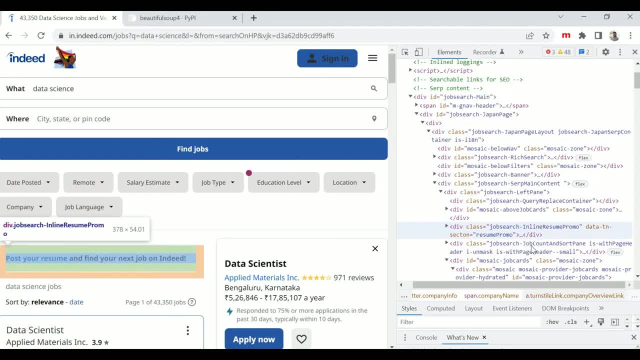 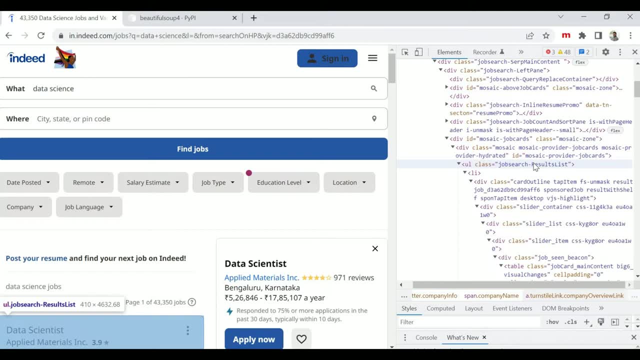 if I'm just coming here like I'm getting like a particular title again, this highlighted part on the left, if I just scroll bit down So you can see that this is the job search list. So let me just scroll down So you'll get it. So there is a list of the jobs if I just go on this job. 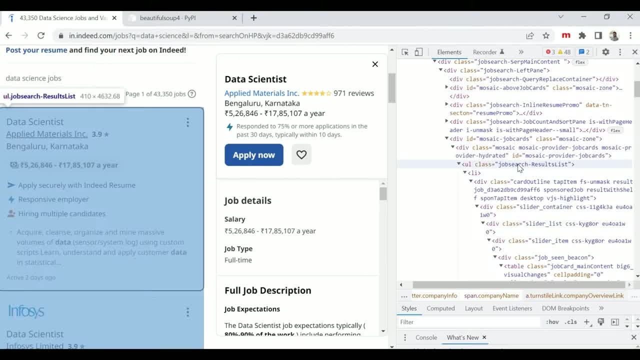 search list. So it is actually having the list of all the jobs. Okay, so this job list we need to access. So let me just go back and first try to convert this whole content to the HTML. So let me just come back to the code And inside of 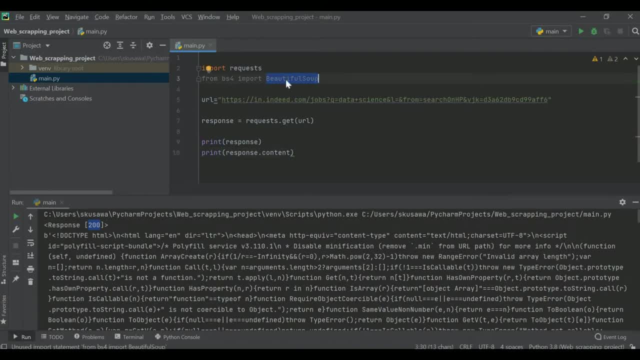 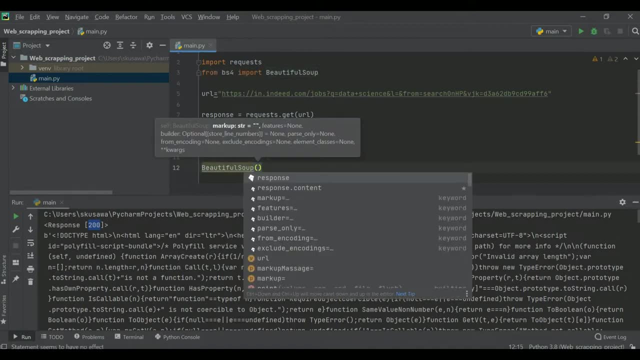 code. let me just try to make use of a beautiful soap So we can pass all content in the HTML format. So I'm just going to make beautiful soap And to this I'm going to pass this response dot content. So this is the response dot content, And I have to mention like what kind of passing I want. 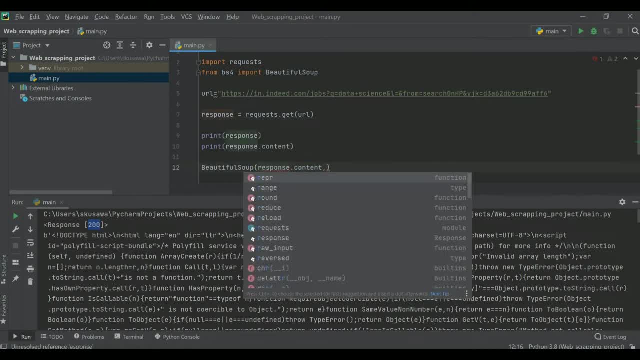 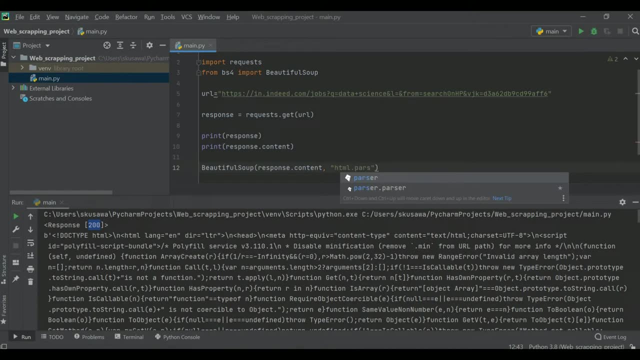 to perform. So let me just type here our response dot content and our parser name. like we want to convert into the HTML parser, So HTML parser. So it will convert the data into the HTML format And you can see the data we are getting. we can make like a page content or something. Okay, page. 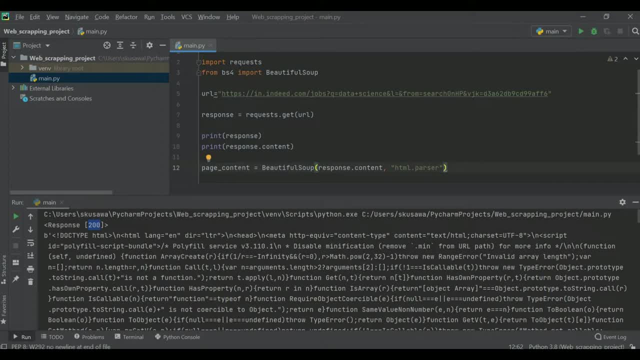 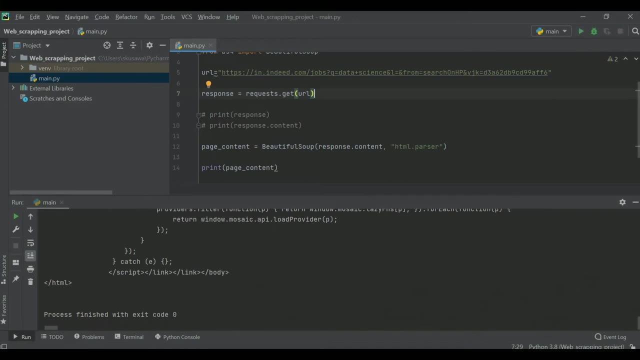 content. and that's it. Now it looks good for me, And let's try to print this page content So we'll be able to see on the console like how we are parsing our all page data in the HTML format. And let's come in this previous one. Let me just run and show you the HTML content. So now you can. 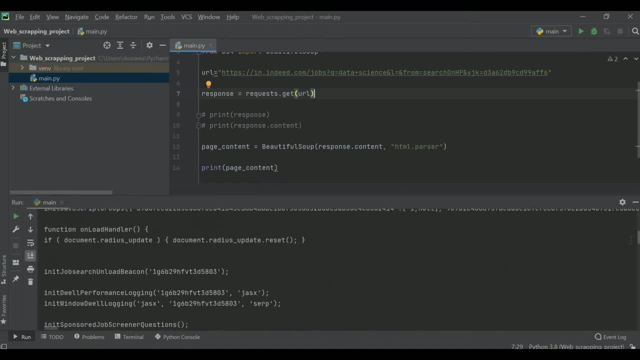 see that we are getting a more structured data. So if you see here, so we have a lot of HTML data. okay, let me just come down. So this is the scripts and these are all the okay. so from here you can see. 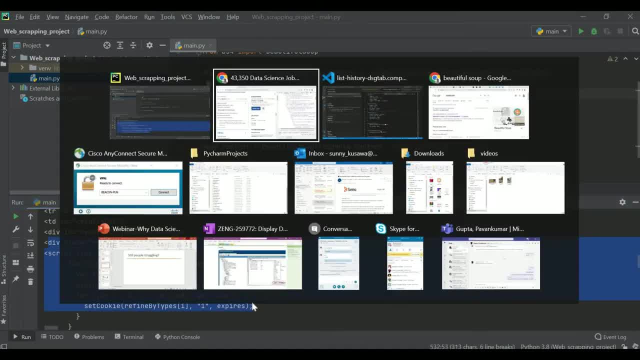 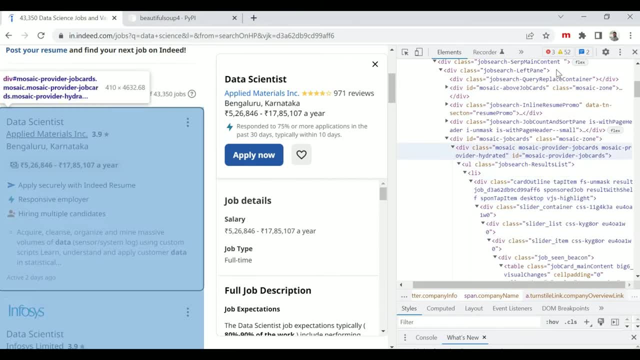 that this is a actual HTML content which I have shown on the site. Okay, so this is the HTML content now we are able to access. So now our data, all the web page content, is got converted into the HTML. we are able to extract that HTML content And from that we have again need to do the 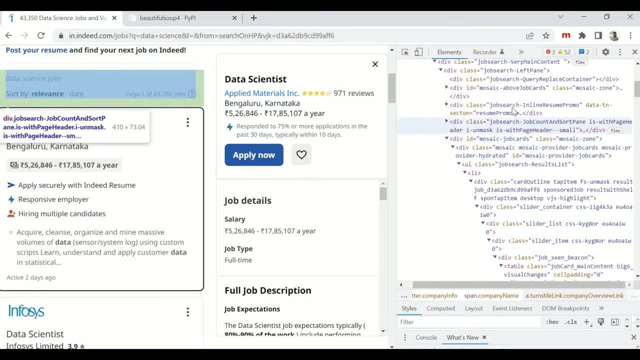 scrapping means we have to face the specific data, we have to face the all the list of jobs And inside of those list of jobs, we are going to face the list of jobs. So we are going to face the list, we are going to face the actual each job. So how you can do that. So let's consider, we want to see 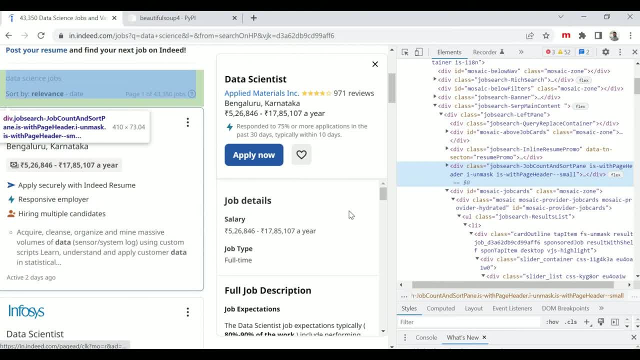 the all list of jobs. So right click and click on the inspect And when you go on the right hand side, once you keep hoarding, you can see that. okay, so this is the job search list, is nothing but the list of the all job. So first we are going to access this one job search list, Okay, 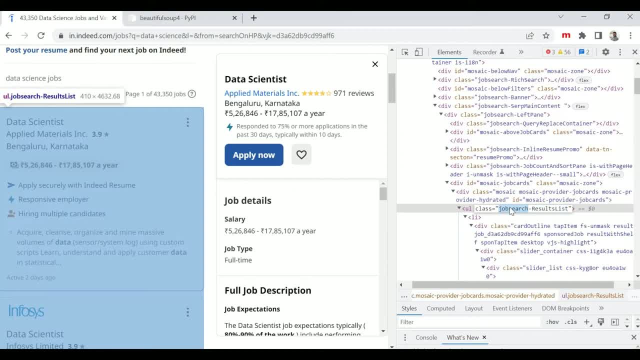 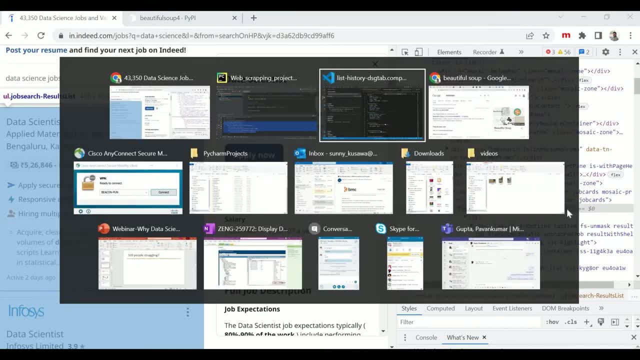 so this is the class of this particular tag, So I'm going to use it. Okay, so if you're using a class, you have to use a dot inside of our code. Okay, so, let me just go in the inside of a code again. Okay, sorry here, And let me just try to access it. Okay, So, from this page. 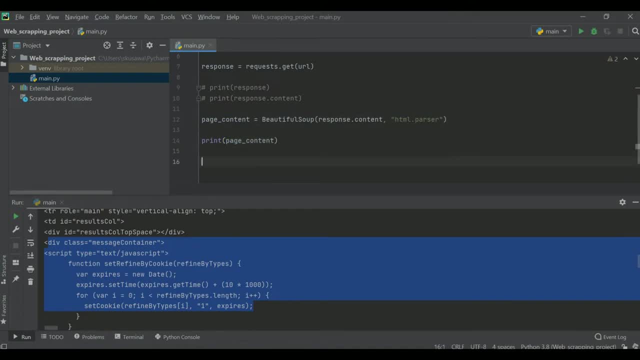 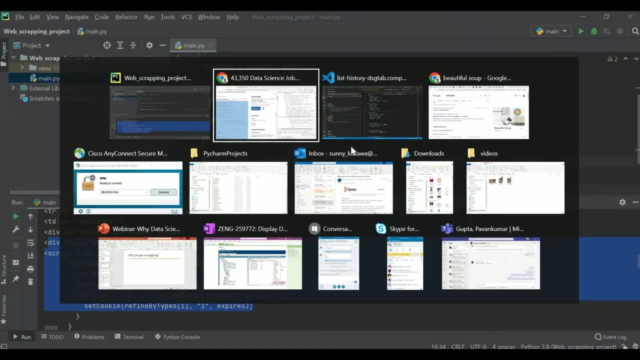 content. I'm going to select only specific interested job list. So I'm just going to say like a page content, dot select, And here we have to pass this particular class we have copied. Sorry, so I again need to go back and copy the class name like a job search list. So this is the class name. 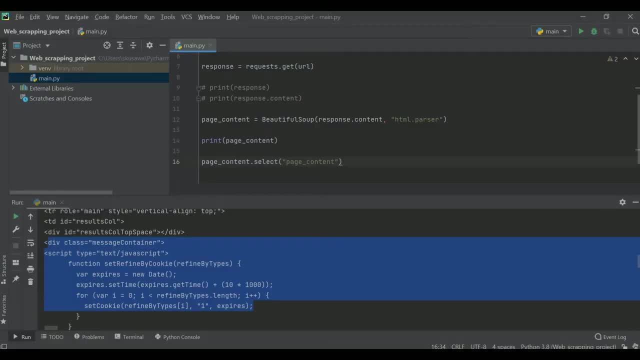 I'm going to copy, Let me just come back and let me just paste it over here. Okay, so it is a class, So we have to use like a dot before it. Okay, so it is a naming clutcher in UI for the CSS. So I just don't want. 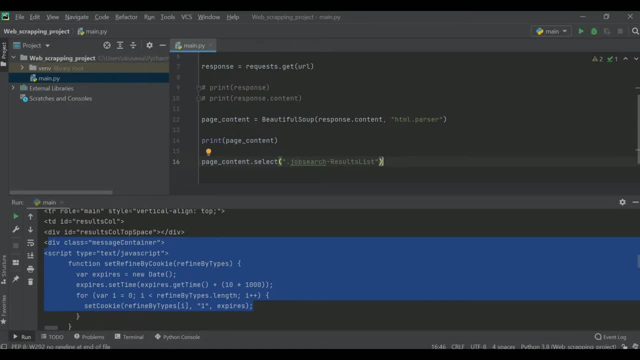 to dig more on this. If there is an ID, we have to use hash. if there is a class, we have to use a dot. So I'm using dot here because it is a class on that particular element and that element I want to access. that is all job list And whatever the content I'm getting, let me just store in one. 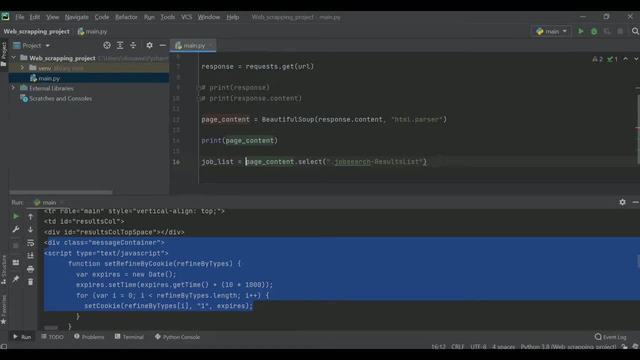 variable and name it like a job list. Okay, so that's it. Now we'll be getting the all the jobs which are available on that page inside of this job list. So this, that would be kind of whole HTML content related to the all the list of. 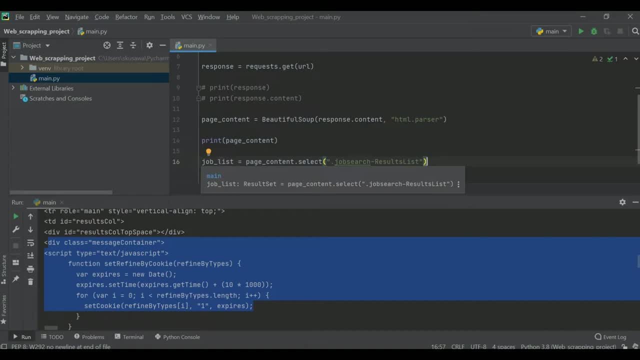 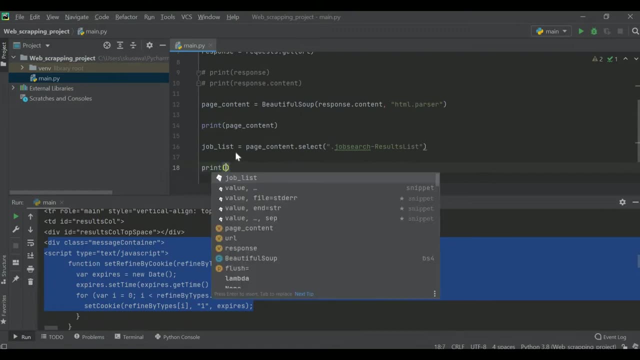 the jobs. So let me just try to run and let's try to print and see like what exactly we are getting. Okay, so let me just go here here And let me say like a print, Let me just try to say like a job. 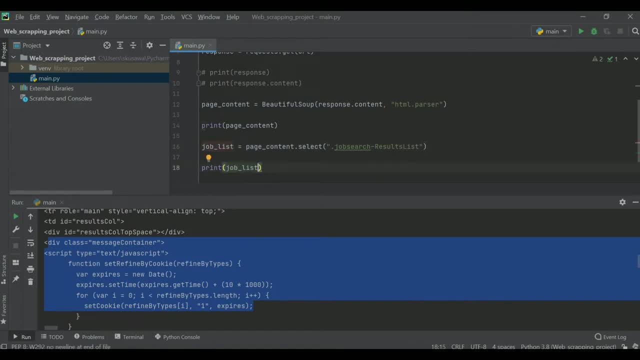 list. That's it And comment this part, Because we don't want to access the whole page and print it over here. We are just accessing the whole page, but we are just interested in the job list, So let me just try to run it. 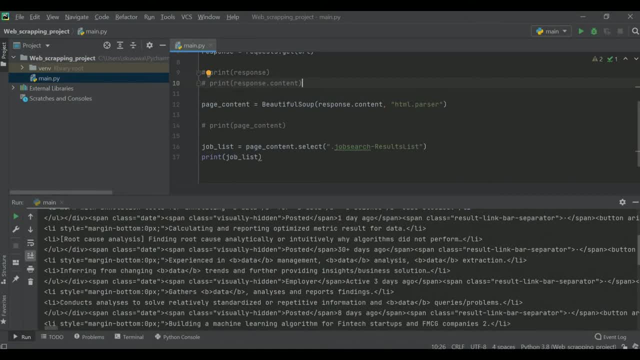 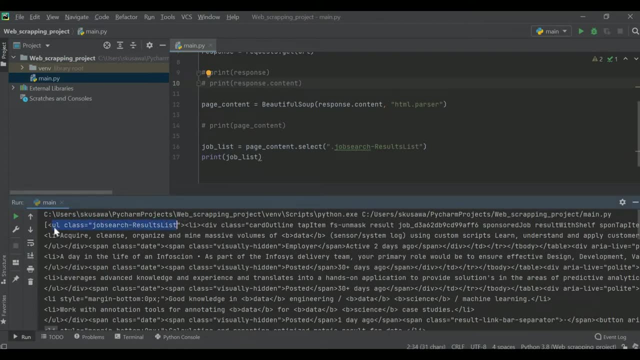 Okay, so here you can see that I'm able to access the only part in which I'm interested in. Okay, so you can see that this is the part related to the job search list And this is the all content inside of this particular tag. Now, inside of this job list, we have the multiple jobs, So we have 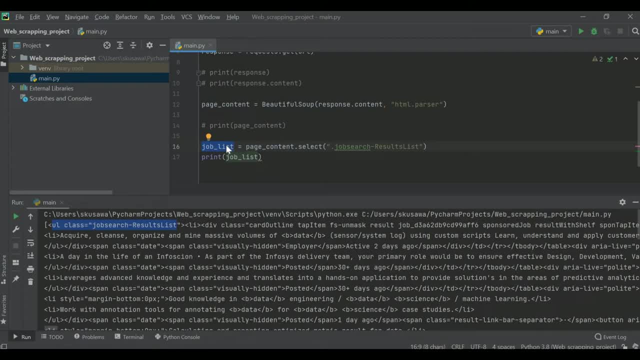 to access each job one by one. So how we can access it? okay, so actually, this page content dot select will give the list of all the elements which is having the class this, So it is actually returns the list. So inside of this job list, we want only this first one tag. Okay, So inside of that we have. 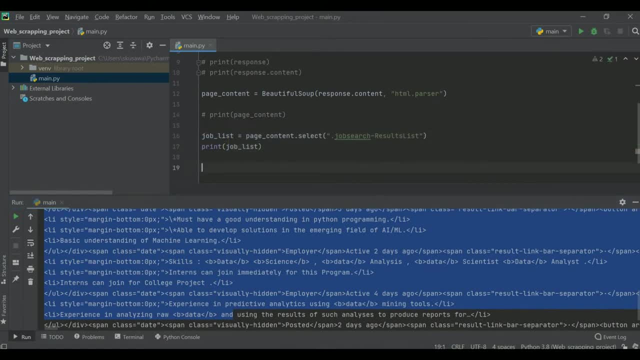 a lot of data, So how we can access it? So it is a list. we can just access it as a zero index element. Okay, So when I'm saying zero element, so let's try to understand what exactly I'm saying. 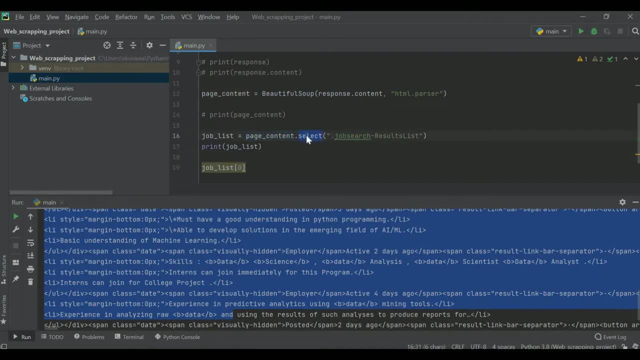 So we have the whole page content And we are also able to access the whole page content And we are selecting the all the elements on this page content which are having this class. So it might possible this class have at multiple places, but we are just interested in the first one. So this: 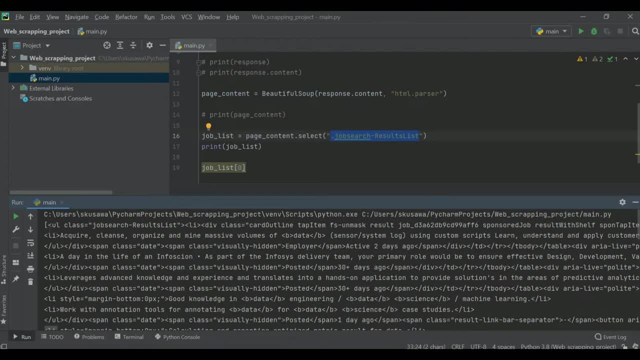 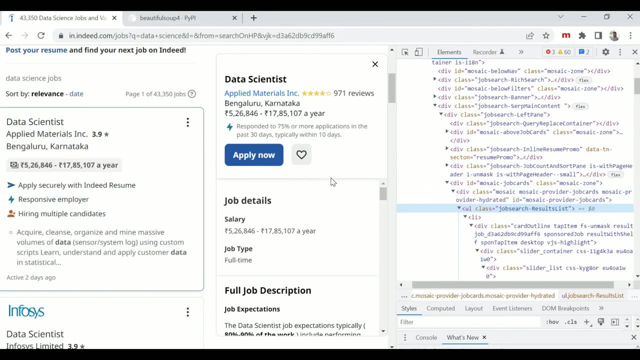 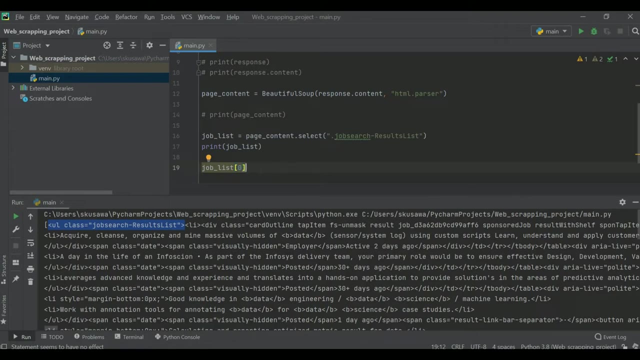 one I just shown you. So this one we are interested in. Okay, so, as I mentioned on the page, so this one we are just interested in because it is related to the job list. Now, inside of that we have the multiple jobs, So how we can access the each job from this particular all job list. So 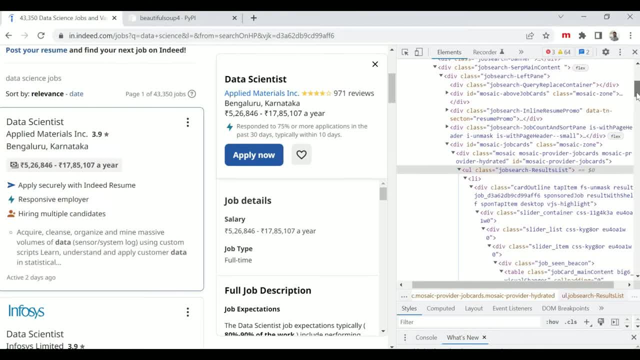 we have to see, like what are all unique identities we are getting for each job based on that we can face. So I'm just selecting this one card. Okay, so this is the one job related information I can just right click and see, like inspect. So when I'm saying that, so I guess it is selected. 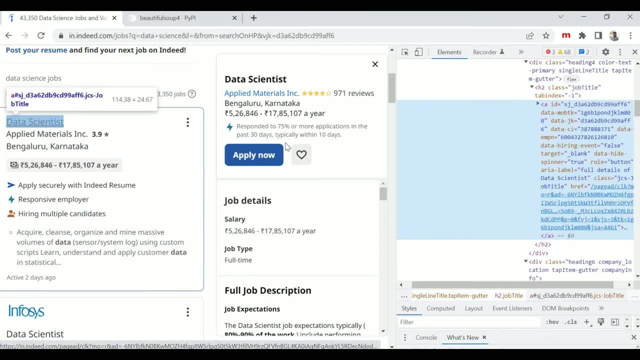 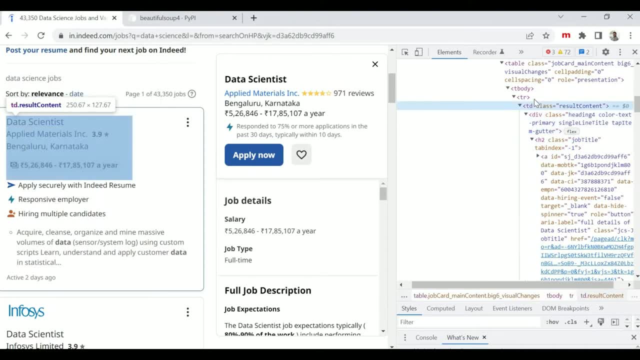 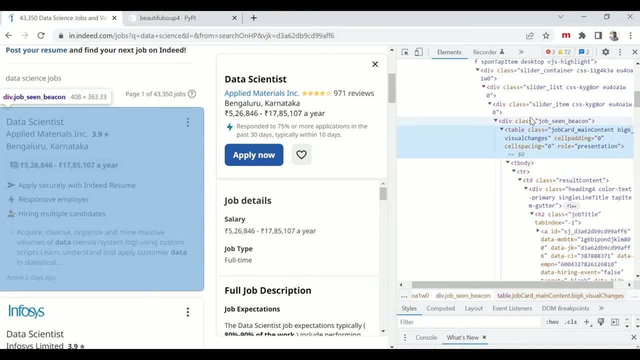 the all this hyperlink. let me just reselect, inspect. it is again selecting. So let me just go to the parent and see like which element or the tag highlighting the whole job details. Okay, so I'm just going up. This is highlighting only half part. I'm just going again up. Okay, so here you can see that. 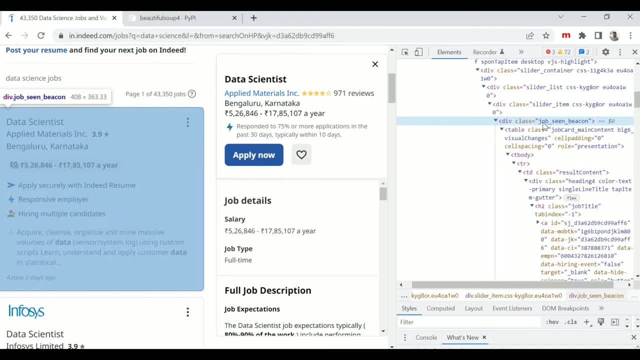 under this deal. I could see like it is having the all job details. Okay, so I just selected this deal And on left hand side so you can see that this is the all content gets selected. Okay means inside of this particular deal, we have the all these job details. If I go to the next job and 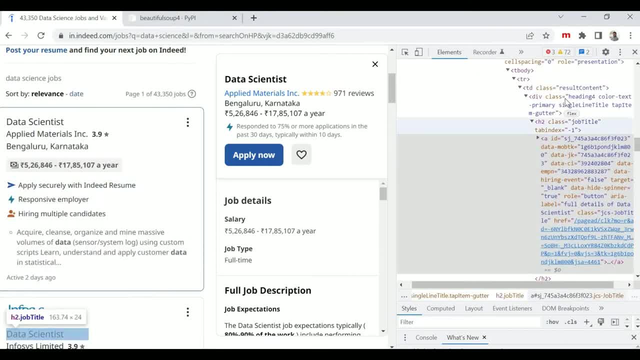 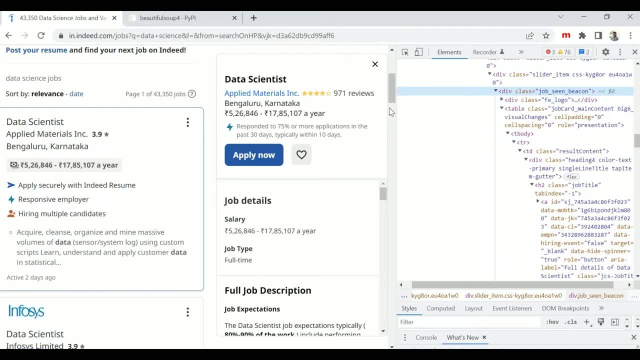 do the same inspect. And if I just go up up here and you can see like let me just keep moving jobs in, You can see that it has selected the second job. let me just scroll bit down so you will get a. 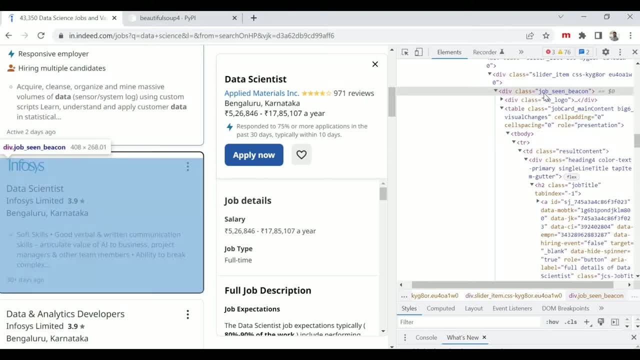 better idea, So let me just go over And you can see that this is the content selected. Now you can see this. all job details are inside this deal, which is having the class like a job scene beacon. Okay, so this information I can use and I can access the all job details one by one. Okay, 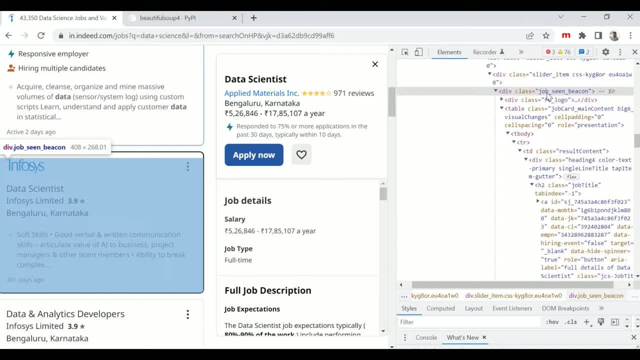 so how I can access it. like already, I'm having the all job list inside of my job list, zeroth location, And from that I can access the all elements which are having the deal and class like a job sit beacon, So how we can write a logic for that. So let me just go back into the code. 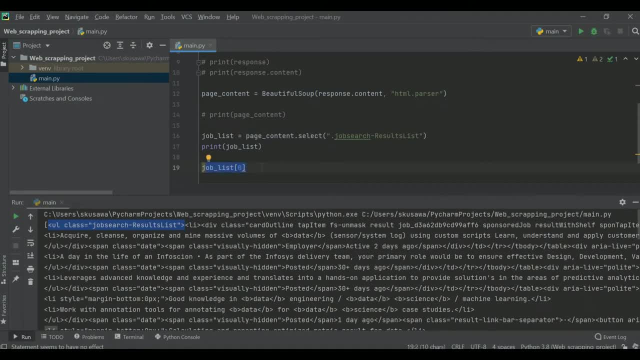 And from this job list means all the jobs. I'm going to access the only those jobs. So I'm going to say, like a find all elements inside of this particular data which is having the tag name as a deal and class name. Okay, so for that we have to pass the problem. 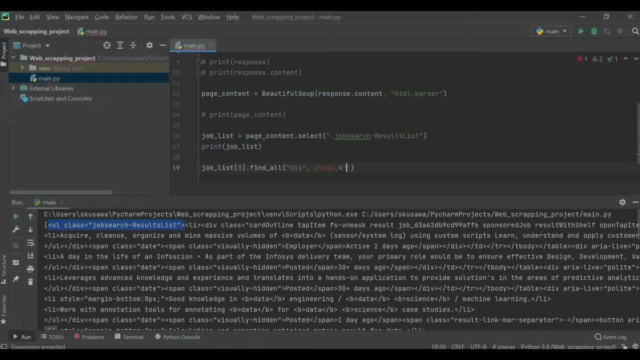 like class underscore equal to. and then we have to pass the class name. so I am going to the page and what is the class name? like a job scene beacon, so let me just copy and come back and paste it over here, okay, so you are able to catch. 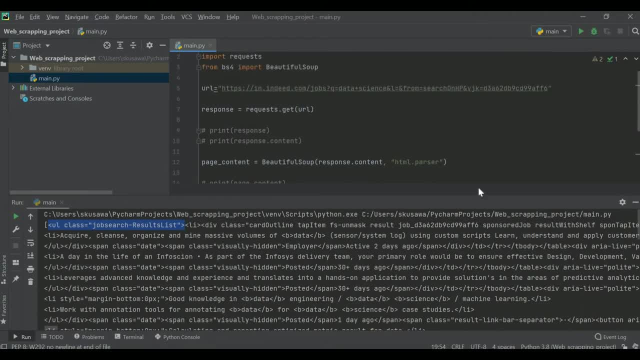 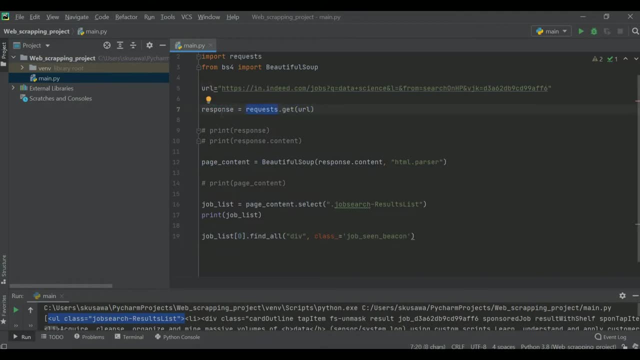 up till now because we are just access the whole web page. let me just repeat for you guys. so let me just maximize the code. we have taken the URL, we have access the URL with the help of a request API and then we have whatever the response content we are getting. we have passed into HTML format with the 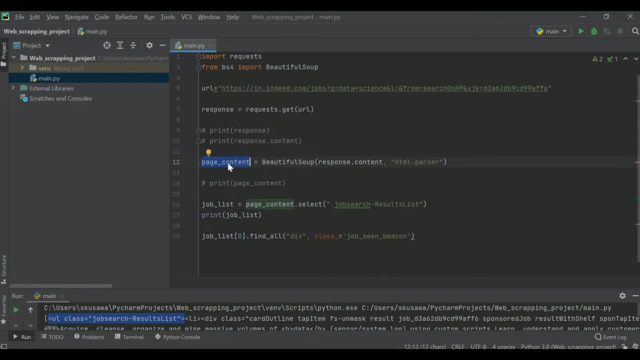 help of a beautiful soap. then we got the all content, HTML content, page content in this variable. from that we have selected the only data which is having the class like a job search results. so it returns a list and from that list we have just selected the first one and inside of that we have the 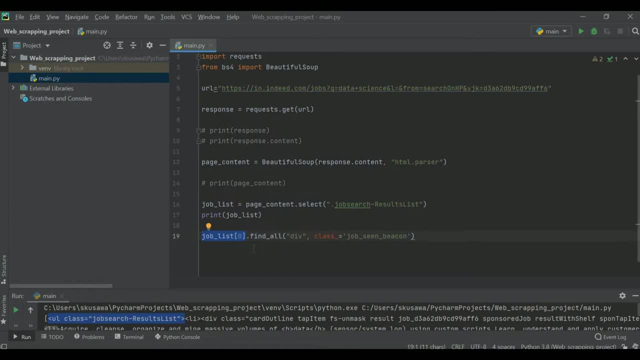 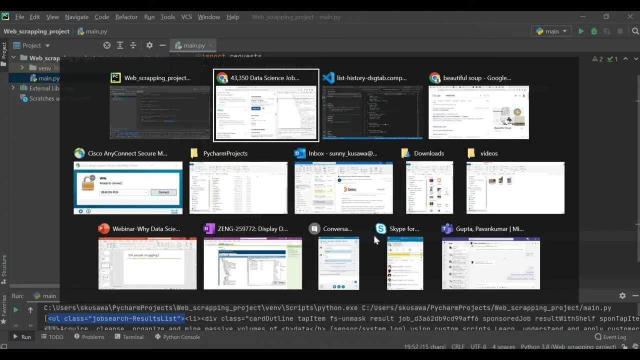 all our job list and from that job list we are trying to access the all the tags which are having the div and the jobs in beacon class. why we have selected this? because each job is available inside of this particular tag with this particular class. okay, so, as you can go here again and see, so each job is having like a div and it is. 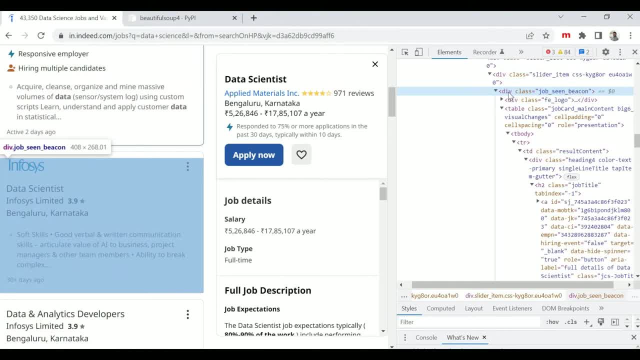 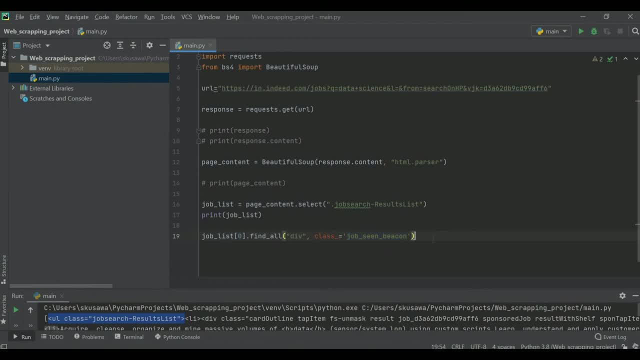 having class like a jobs in beacon. so if you access this, then again inside of each job, we will be able to fetch the job name and company name and all those details. so let's come back over here and let's try to access this all job list. 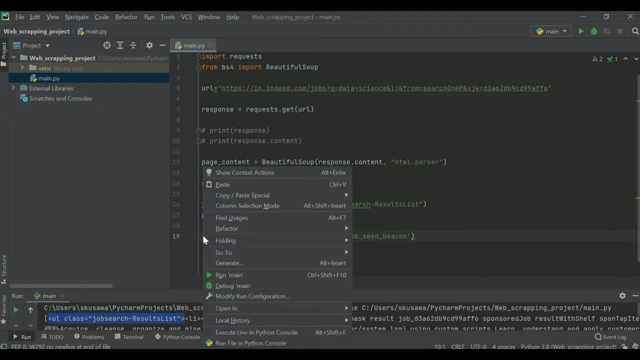 and store this job list in one variable and name it like something, like a jobs. okay, so just say: look, just give me a count once here let's begin. let's say like one variable jobs, and inside of that will store this, all the. this would be the job. 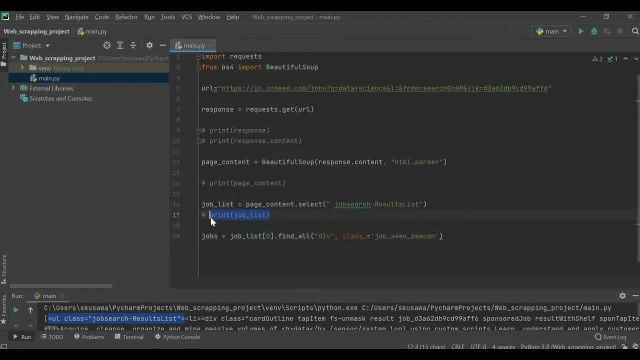 list. okay, if you want to again print and check, then again I can comment this and let's come back, copy past and just print this jobs and let's see the results. okay, so now we want to be able to see this. we will be just able to see the all the. 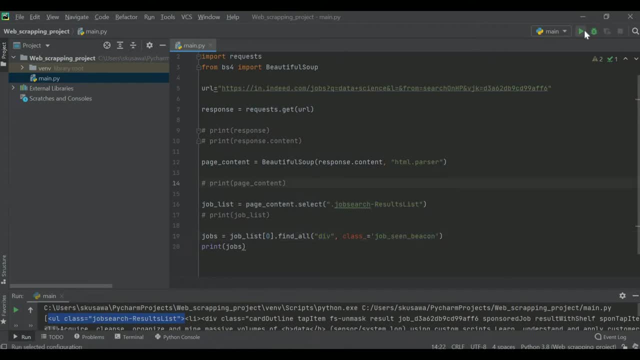 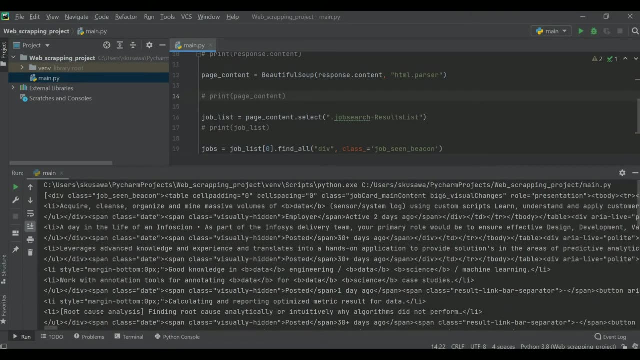 items, which is having the div and the class, like at this. so let me just try to run it. okay, so it's ran successfully. let me just go on the top so you can see that we are getting like each class list like a job class would add multiple job. 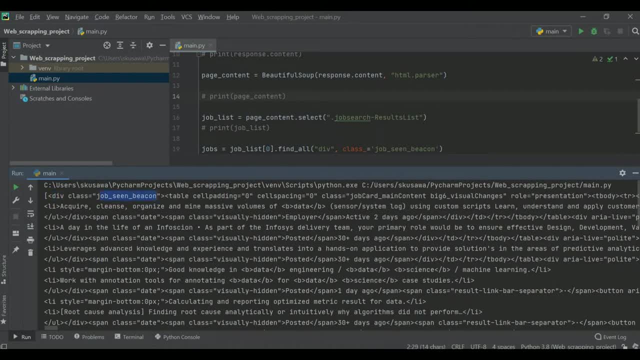 list like three to four. we can use the jogs just to see it. okay, so let me just a each div which is having like a jobs in beacon as a class. okay, so there would be multiple, so let me just try to search and show you. so let me just select and say ctrl f so you can see that i'm. 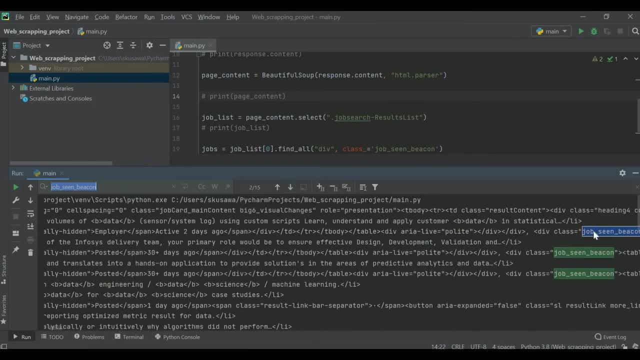 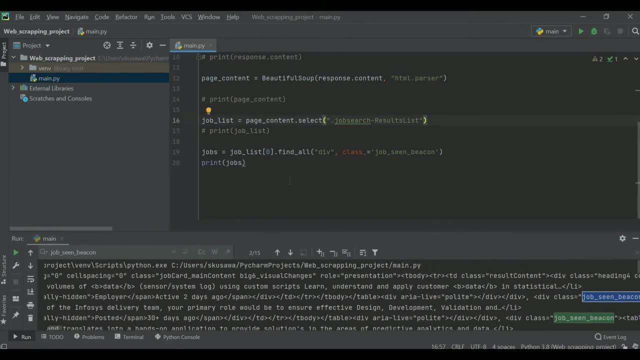 getting the 15 job details if i just click next so you can see that div class and it is having the class name like a job class beacon. okay, so we have the 15 job details available inside of our job list and that job. each job details will try to fetch, so for that we can write a simple for loop. 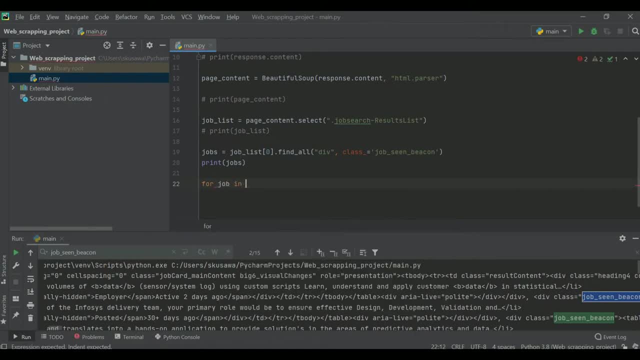 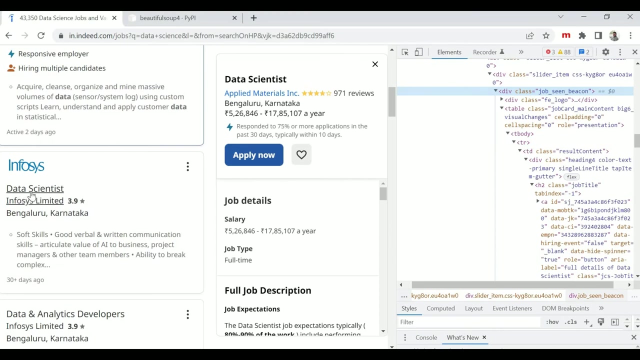 so i'm saying like a for each job inside of this particular job list. i'm going to access each job and from that job we are going to access the specific fields. so what we were interested in. so let me just go on to the page and now you can see that each job is having like a job title and 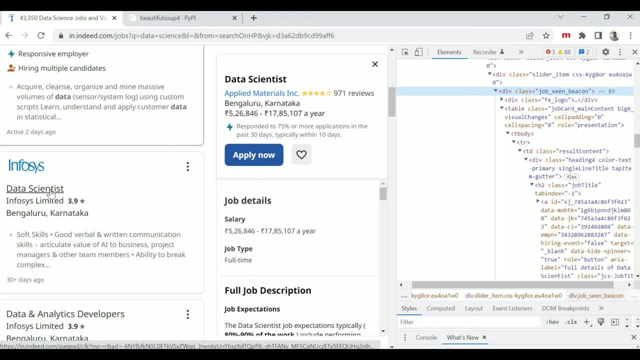 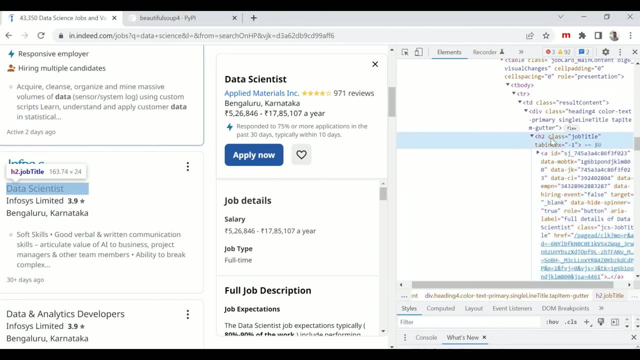 the company name and location. so let's see like what exactly this company name is, so or that this particular job title is. so let me just right click and inspect, so here you can see that this particular job too, i could see like it is available under the h2 tag and it is having like a job title okay, so you can see that it has having. 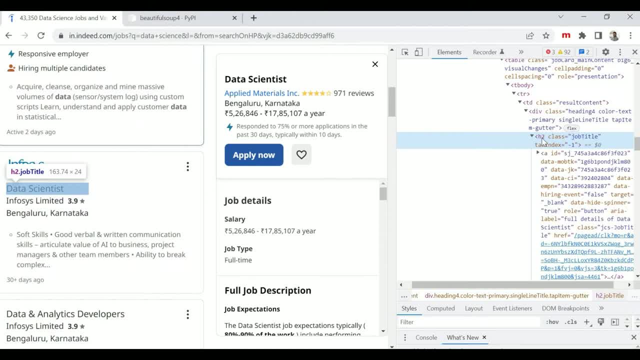 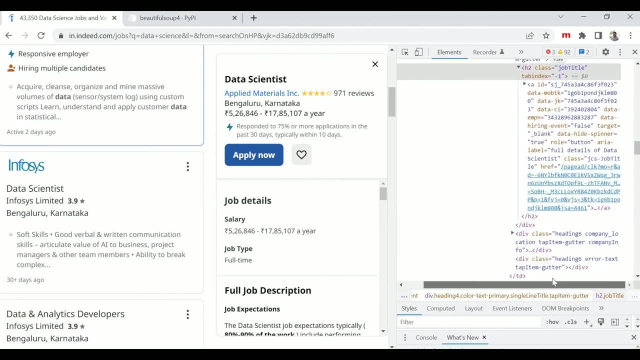 like a job title as a class name and tag name as a h2, so i can, with the help of that, i can access inside of each job whatever the h2 tag, which is the class name, job title is nothing but the title of the job, because inside of that we have here the job title. so let me just go on to the page. 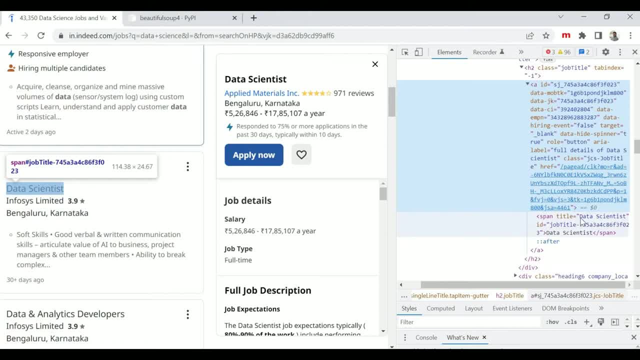 so here we'll be able to see like: this is the title. okay, so you can see that this is a, this is the title like a data scientist, okay. so here it is okay, so this is a data scientist title. so what i'm doing: i'll access this h2 with the class name, job title and inside of that, whatever. 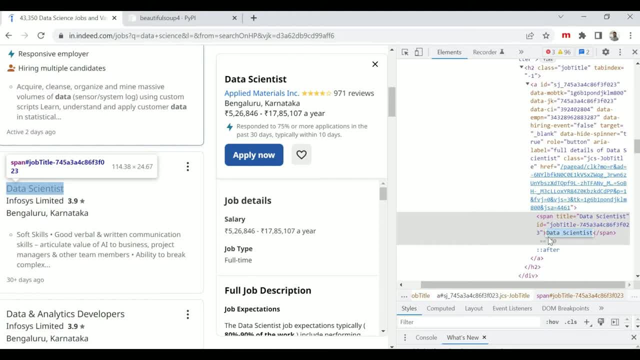 the text content i am getting. okay, so these are all tags. i'll just access the text. so this is the text. like a data scientist is a text, so i'll be able to fetch. so if you just go and check for another job list, right click and inspect another job title. so this would be. 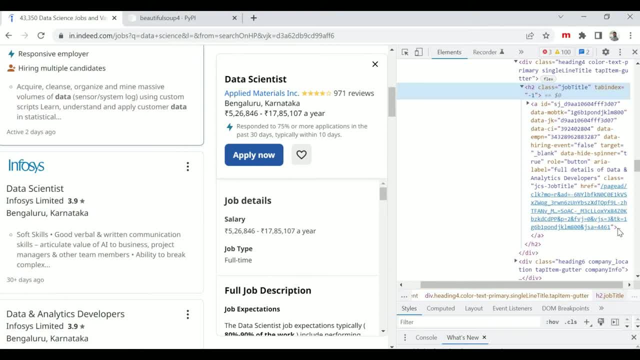 structure like h2, job title, and inside of that we have the text: okay, so let me just expand it so you can see this is the job data analyst developer. okay, so this is data analyst developer. so i am going to access each h2 tag with a job title class and from that i am just going to 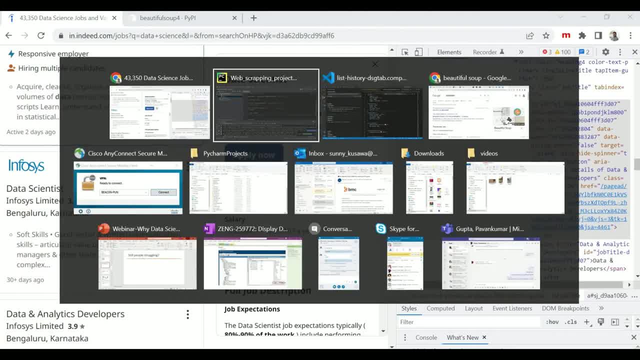 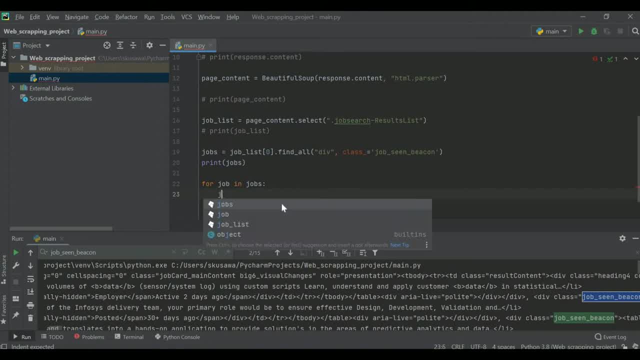 extract this text. so let me just go and show you. so i'm just going back to our code and from this each job, what i will do, i'll try to fetch the particular h2 tag. so let me just say, like a job, and inside of that i am going to find h2 tag. whenever i found the h2 tag, i'll check that. 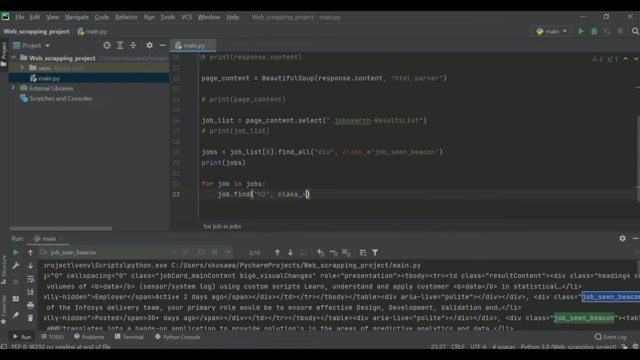 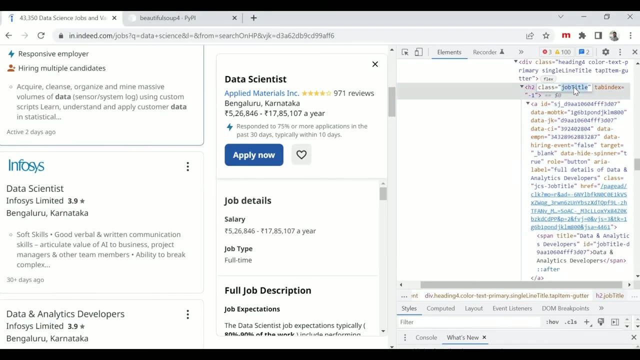 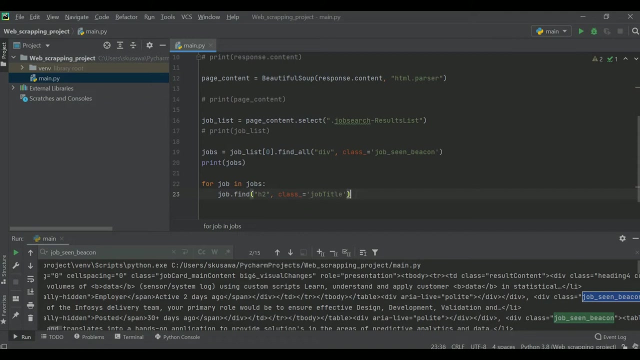 whether its class is equal to okay. so let me just go and see like what class it is okay. so its class is like h2, job title. so let me just copy this class, come back and paste it over here, so all h2 tags with a job title and inside of that, whatever the text we are having. we want that text. 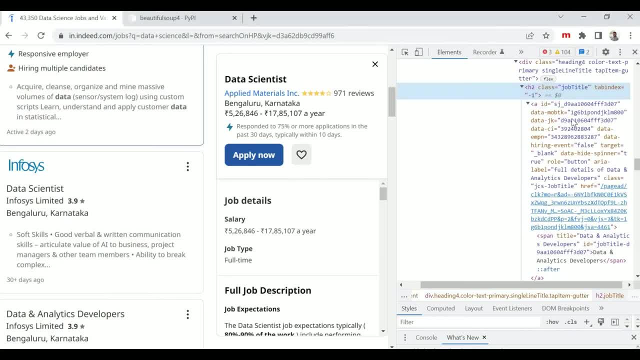 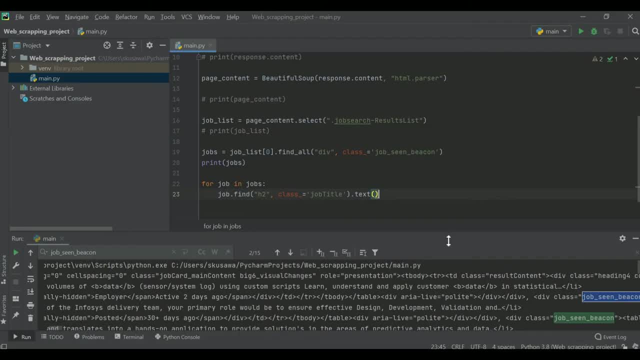 and inside of that we have the text. so inside of that tag, if you see there are multiple tags, but it will ignore all tags and it will just select this text, okay, so we are just interested in those text. so let me just go and access this text and let's store this value in one variable name. it 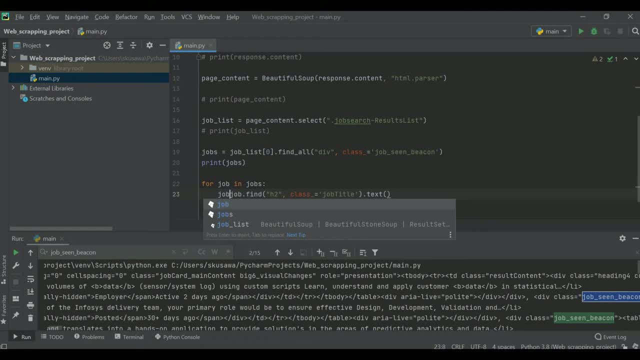 something like a job title, okay. so let me just say like a job title equal to this. okay, fine, and we'll try to print, so we'll get that all for all 15 jobs. what are all the job titles we will be able to see? so let me just say like a job title and that's it. okay, so hope you. 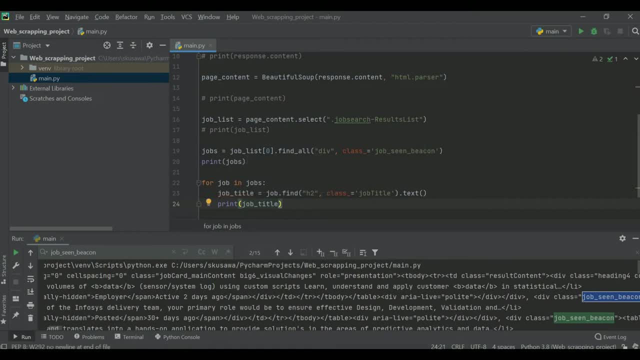 are able to catch up. like we have selected the all job list, from that we have selected the each job and from each job now we are trying to access the job title and all those details. so first of all, we'll just try to access the job title from the job list, we'll select each job and we'll access. 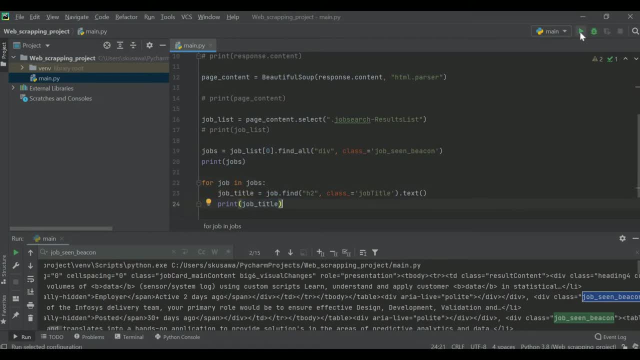 the job title. now let me just try to run and see like we are able to access the job title or not. so let me just comment this: we don't want to print all the raw content now. we are just interested to printing in all the job titles and let's run. okay, so we got some error. so it is. 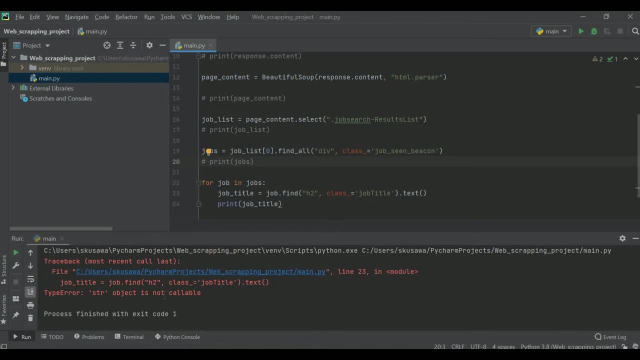 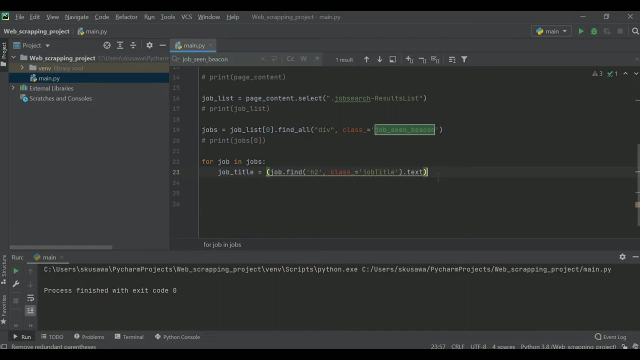 saying: like a string object has not callable. okay, so we are getting some error, because might be we are doing some mistake. so let me just check what exactly it is. okay, let me just try to run now and let's see. okay, so it is running fine. so let me just try to print and let's see. like our all job. 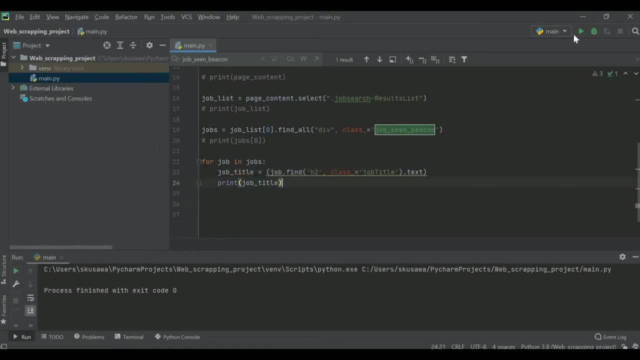 titles. so that's it, and let's good, let me run and show you the all job titles. okay, so you can see that we are getting the job titles of all these jobs available on that particular page. now, this similar way, we can access the all other properties. so this is just like a job. 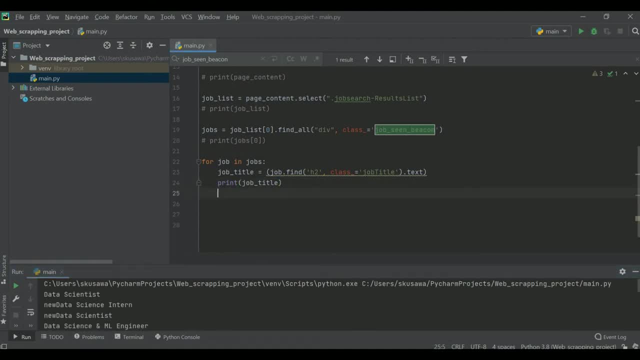 title. so similar way i can access, like other details. so i can go for the next field, like a company name or something. so for accessing a company name, so let's go back to our web page again and here on web page we are getting the job titles. so let's go back to our web page and let's 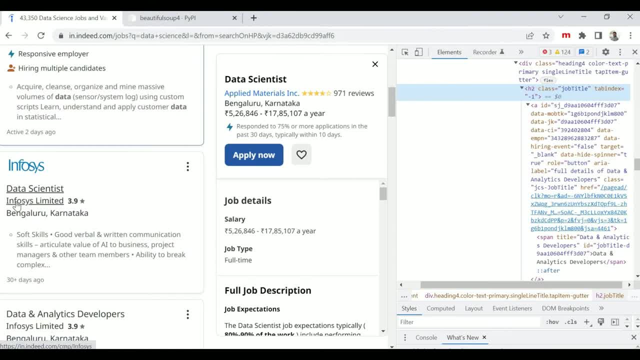 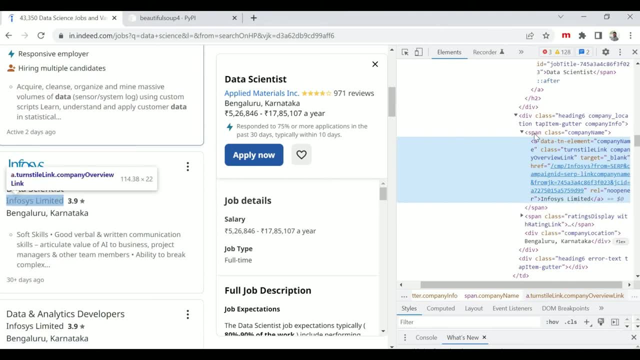 see what we have to search for: the company name. so this is the company name, like infosys limited. right click, inspect and see like what are all details available for that, so you can see that infosys. so i could see like this span: okay, so there is one tag span inside of that. we have the. 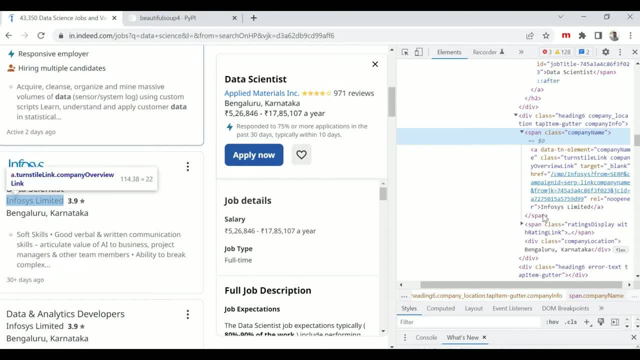 company name and if i just select, and inside of that i'm having the text content like infosys limited, i'm having one anchor tab and inside of that infosys limited text is there. so if i just select this span tag with class name, company name and fetch the text content like infosys limited. 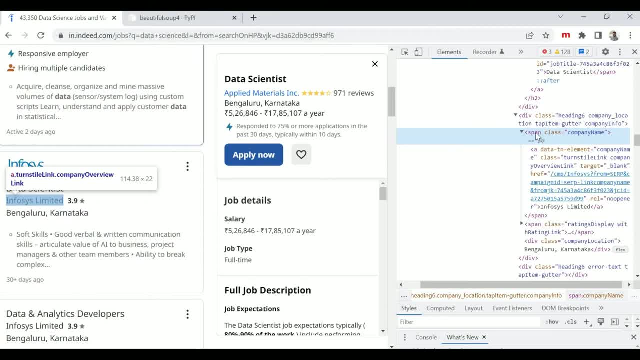 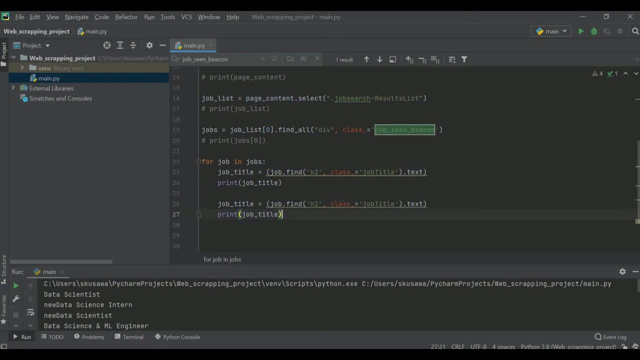 inside of that, then i'll be able to access this company name. so let me just try this strategy. so let me just copy this company name class and go back and search inside of this span tag, so inside of each job. so similar way i can write a code like: let me just copy this and paste over there and let 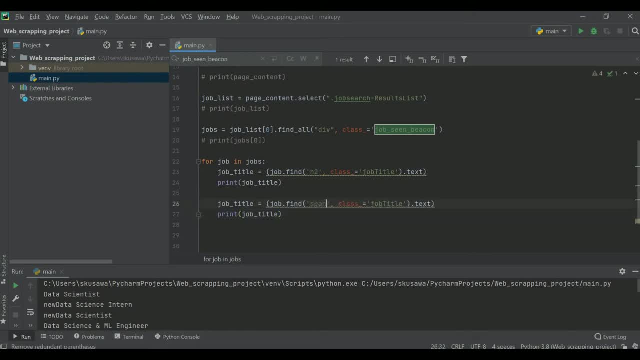 me try. like our tag name is like span and our class name is whatever i have copied, so i have to go back and copy it again like company name. i'm copying, coming back, paste it over here, that's it and let me just rename like a company name or something. okay, so let me just say like company. 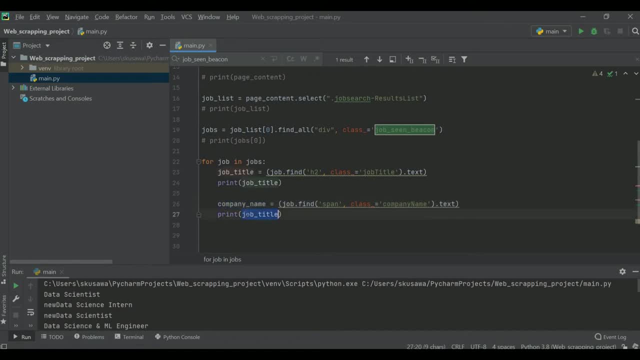 name and let me just paste it like this over here. okay, that's it done. so we'll be going into the each job and we'll finding the span and inside of that span tag, if you find the class name this, fetch it and get its text. that would be your company name. okay, we don't need this extra bracket, so let me. 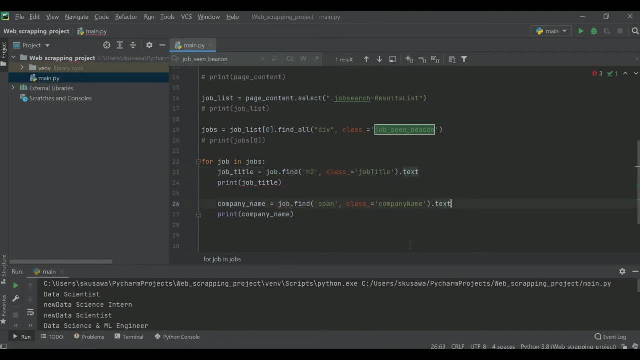 just remove, so we'll it will ignore all the warnings. okay, that's it now. code looks clean. let me just try to run it. okay, so we'll get a printed job title and company name. so if i just go above so you can see that this is the job title and opening is in the applied material science. 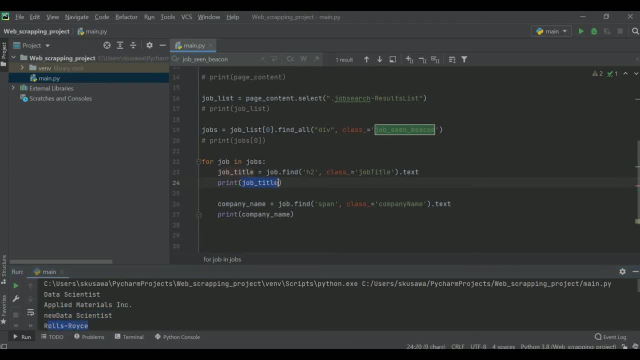 this is second job title and this is the opening. so let me just, for the identification, let me just add it like a text so we'll be able to catch it betterly later on. so let me just put it like this, so it will print like it is job name, it is company name. we'll get a clear idea, so that's it. 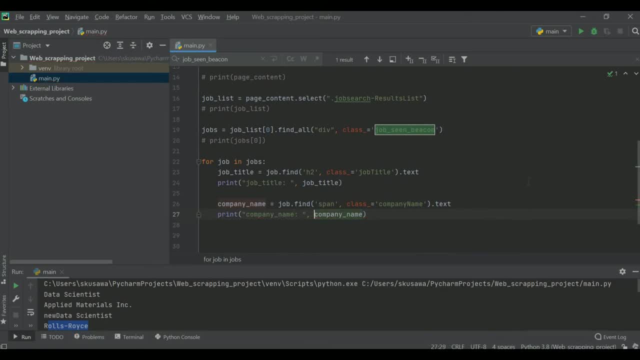 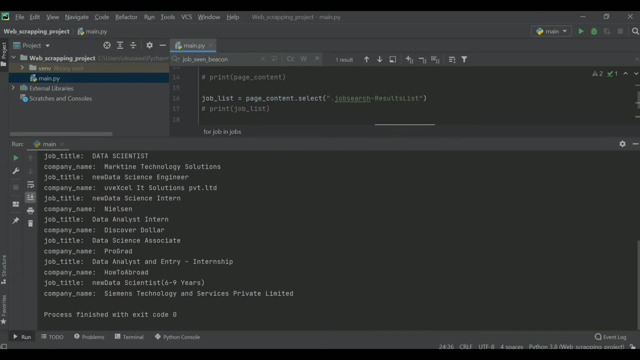 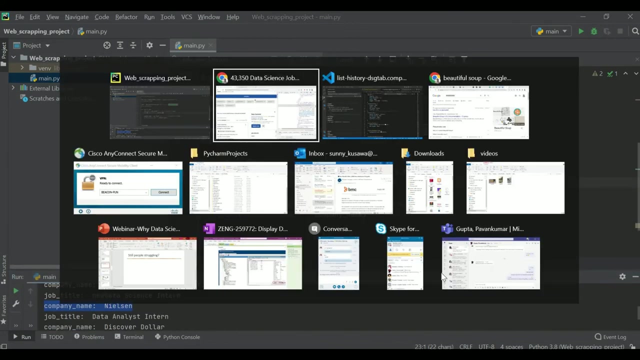 we are looking good and that's it. okay, let me read and show you the clean view. so let me run and you'll be able to see the all the job titles and company name. okay, job title, company name. this is the job title and company name now. if you want to fetch other details, so let me just go back on the. 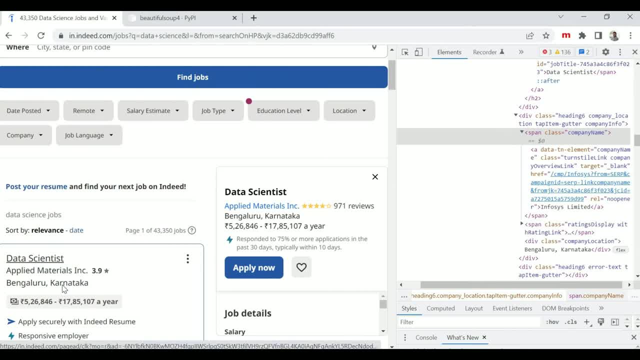 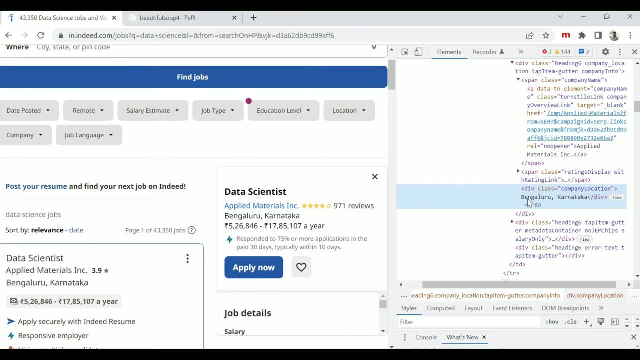 page and if you want to face like this city so you similar way, you can just right click in: so this is the company location, so i can see like this is the inside of div. if i apply for this class, for each job i'll be able to face the city details. 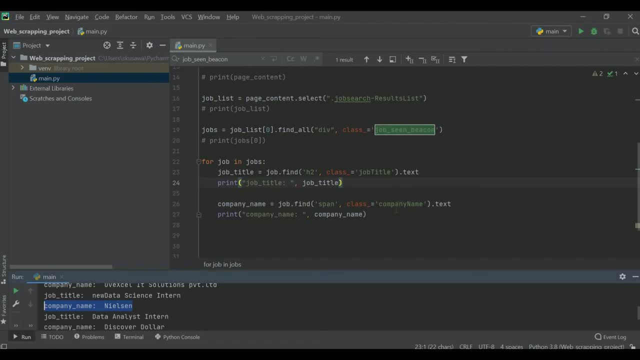 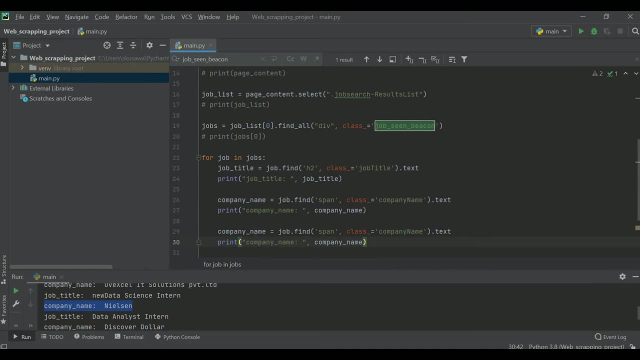 so let me just copy this and go back here. let me just copy paste this structure similar way, okay. and now i'm looking for like a location. okay, so let me just type like a location and let me say like here location, again print location, and inside of div tag we are having: what is the property class name? it is class name, is like. 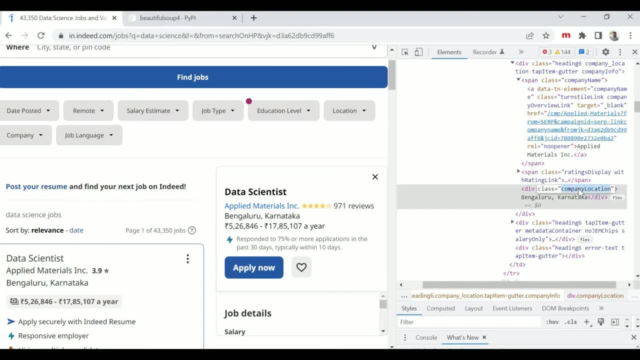 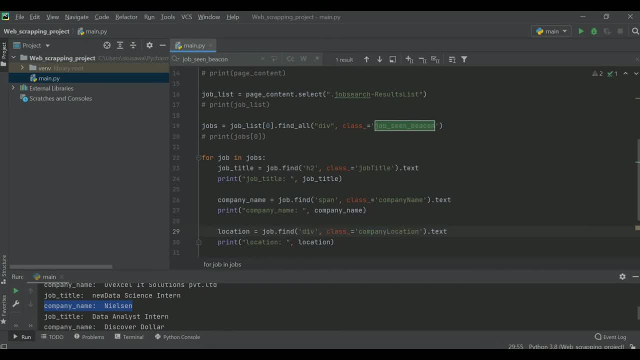 inside of div. if it is a div tag and it is having like a class name as a company location, then put it over here in each job. it will find all divs with a class like a company location and it will fetch its location. okay, and let's try to print and see the results. so let me just go and let me just 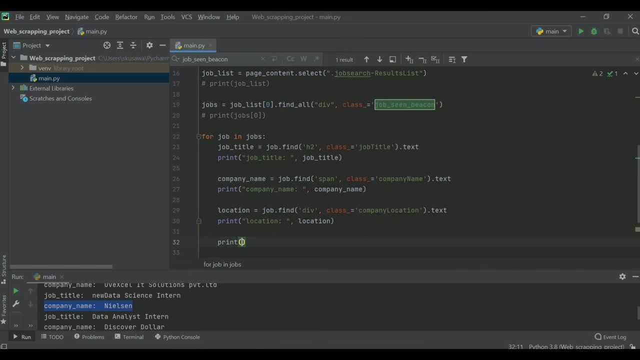 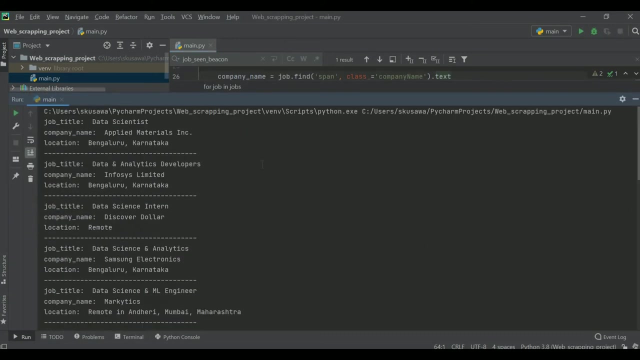 print one blank line here so we'll get the separation, okay. so let me just say like this: okay, looks good, let me just try to run it. okay. so now our out is ready. so let me just go and show you. okay. so here you can see that we are able to fetch job. 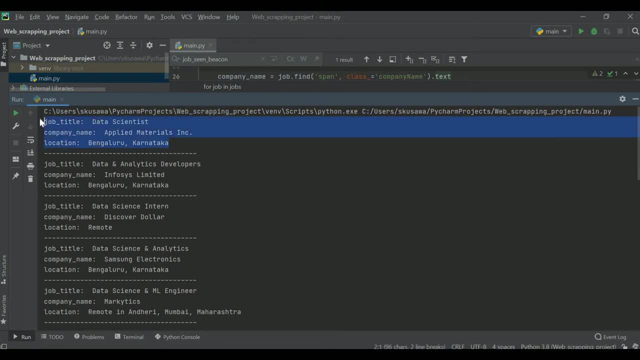 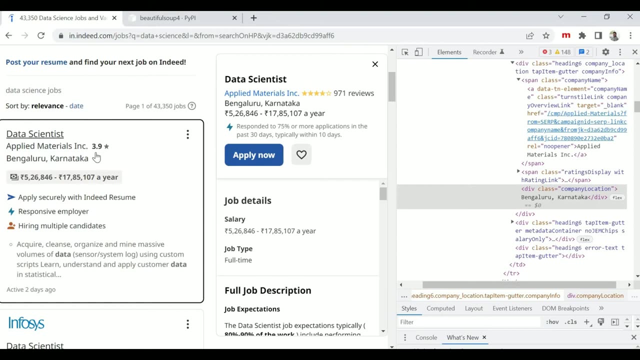 title, company name and location of each job. so this way you can fetch any information related to job. so it is not related to job. you can go to any page. you can just right click, inspect, find the appropriate tags and its classes and with the same method we will be able to face the each content. 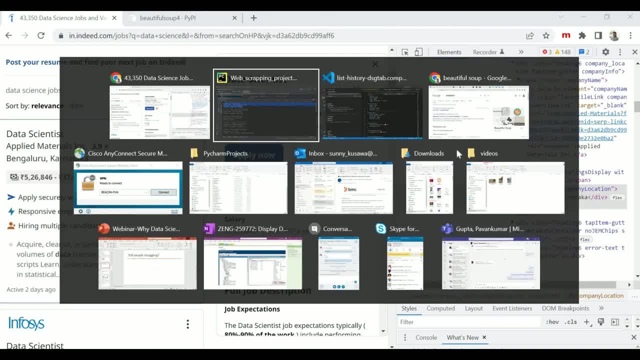 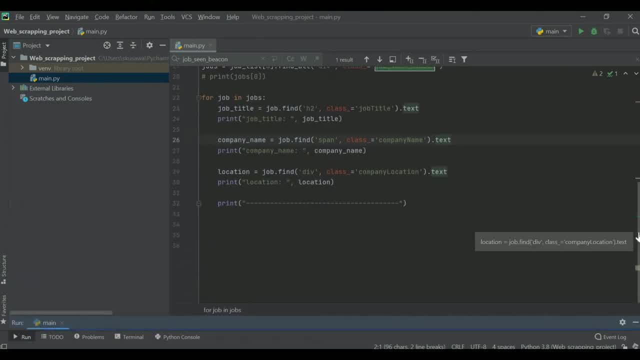 its value on your python code and this way you will be able to prepare the data. so now you are saying, like we, it is fine, like we are fetching all data, but how we can create one data set simply so for that you can, uh, just simply add this all data inside of one list. i would say: 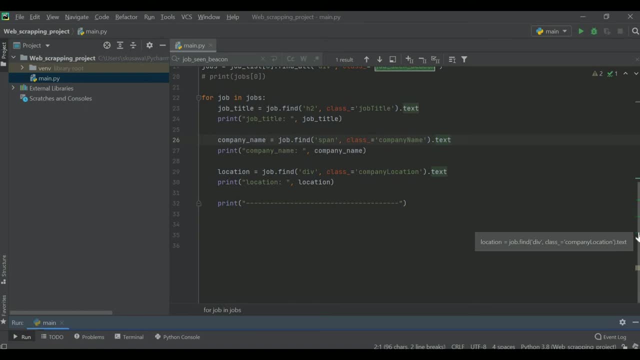 append inside of one list and then you can just from that list you can create a simple csv file, or you can convert that list into the pandas and you can do your job. okay, so let me quickly show you guys like how to do that. okay, so for that i will just create one simple list on top of this. so 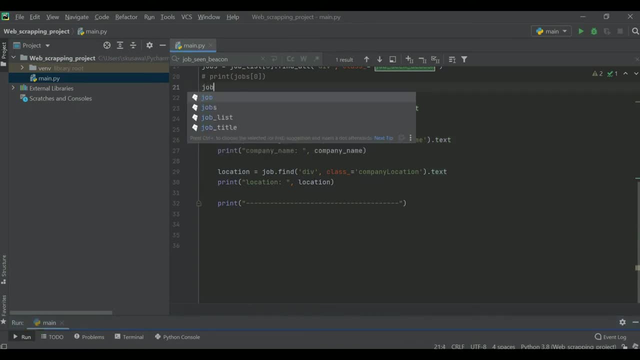 let me just go and say like a job data, something okay. and let me say, like it is a list, okay. so i'm created list with a job data name and inside of this list i'll keep appending all this data. okay, so let me just say: like a job. 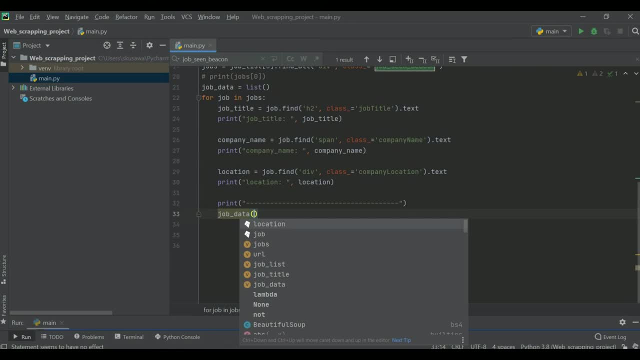 data, and inside of that i'll add, uh, all this content, so i can add this all content as a list, uh, as an element, so i can just create, append- sorry, inside of this i'll just append data and inside of that i'll pass the list. so first will be my, like a job title. 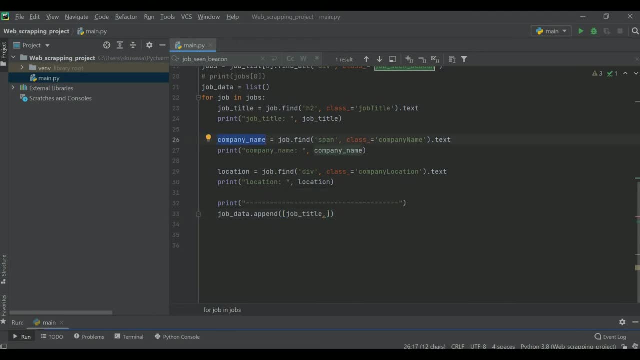 and next would be my job- uh sorry, company name. okay, you can select as many field you want. okay, so you can extract all this field and each field you can push inside of one list and then later on, from that list you can create a file, or you can create a simple pandas data frame, as you wish. whatever you want to do with that data. you can do it okay. so i just start it from here. okay, so i'm going to give you a chance to um. so if you type um right at this point on the top leftml, positph her and then you'll be to the top left every twolect who will post her inside any field if that's the field you want. okay, so you can use as many fields as you wish. whatever you want to do with the data, you can do it okay. 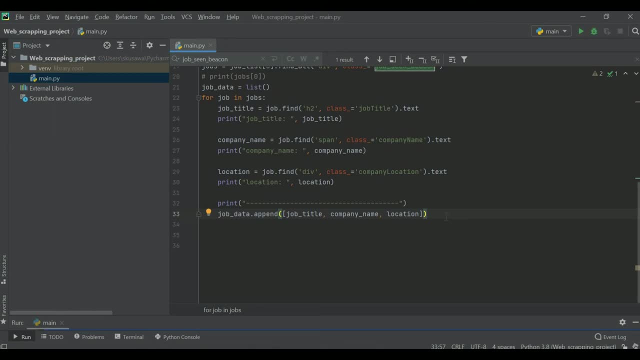 just giving you one simple example, like: if you want to collect this data and save inside a file or create a data frame, then how you can do it. okay, so once our all job, we have iterated through all job and we got the all data inside of our job data list, so from that again you can create a pandas. 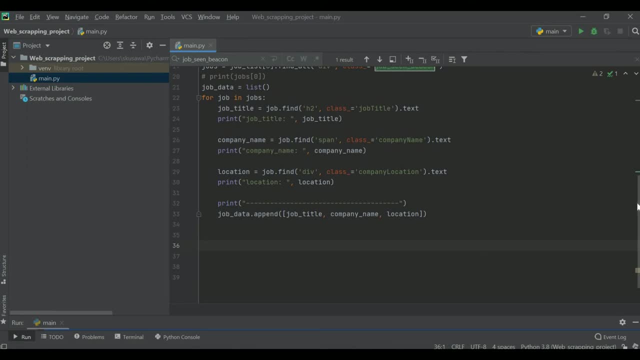 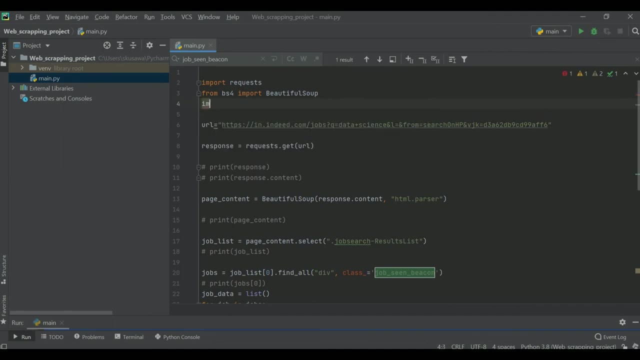 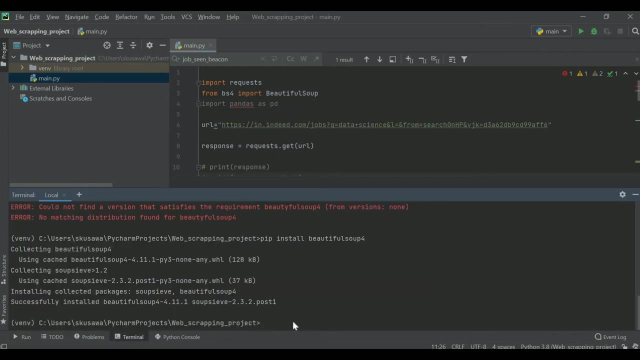 data frame. okay, so how you can create like for that. we have to, i guess, install a panda. so let me just see like if pandas is available. so let me just say like a import, sorry, import pandas as pd. okay, so i could see like pandas is not installed, so let me just quickly install it for. 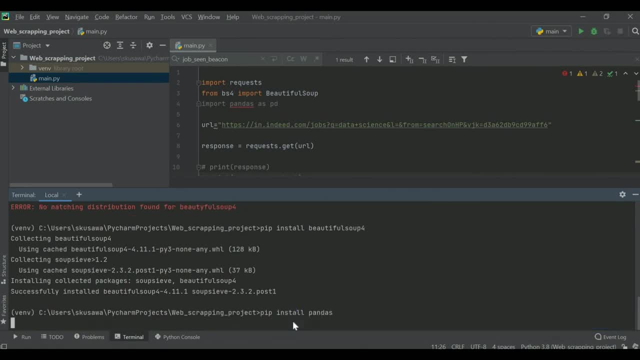 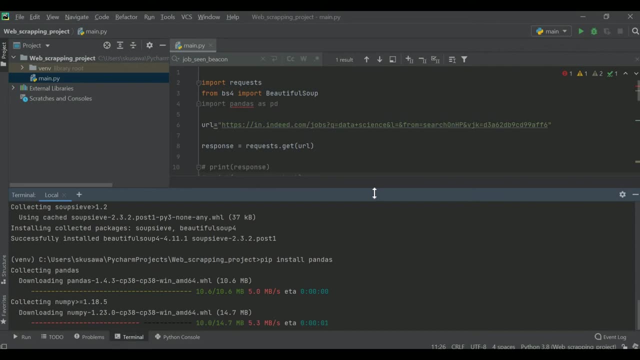 you. okay, so pip, install pandas and once it install we'll try to create a data frame from the list. okay, so it is downloading some required packages like numpy and all pyth, and once it install we will be ready to use this pandas library. okay, so it is taking time. okay, so now here you can see. 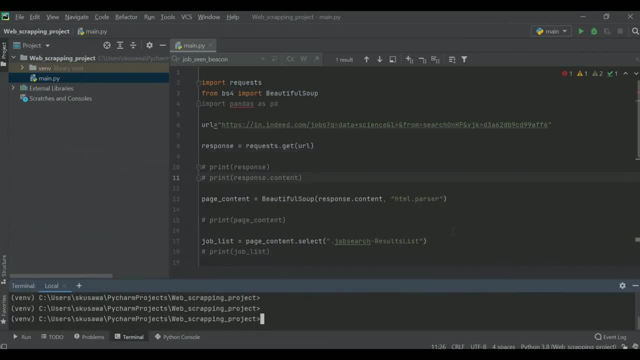 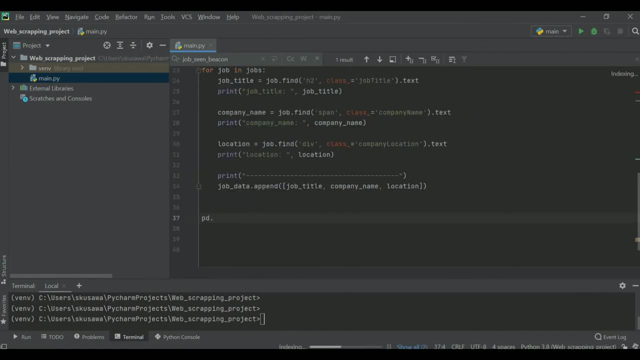 that our packages are installed. so let me just say, like, pandas is not installed, so let me just install. so now let's go back, okay, and let's try to access it, okay. so i'm going back. so i'll say, like a pd dot, i'll make use of a data frame from pandas library and i'll create a new data frame. 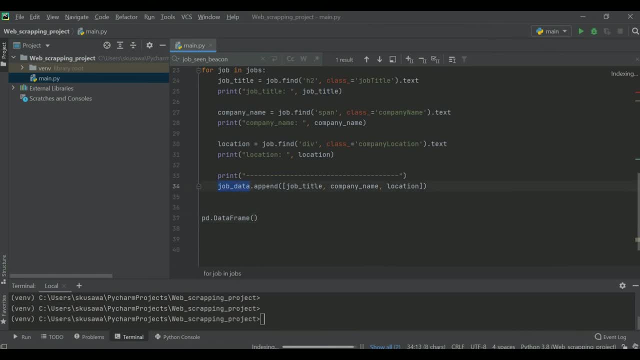 by passing all this data. okay, so this is my job data, all the list of data, and if you want to pass the column names, then you can just mention here like a columns and you can pass all column names as a list. okay, so if you want to give this, you can give the same. 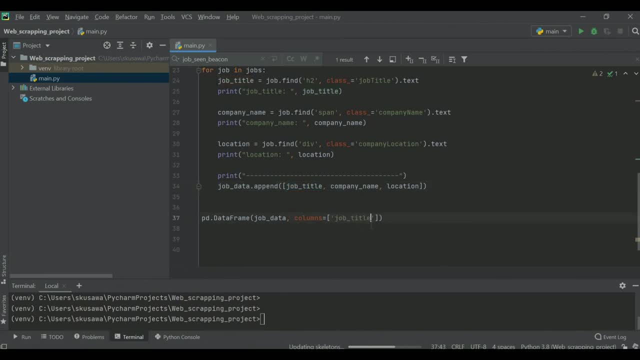 as a column names, like a first column would be like a job title, second column would be like company name and third would be like a location. okay, so, okay, copy paste job. fine, so we are creating one data frame where we'll push all the job details with these three column details. okay, 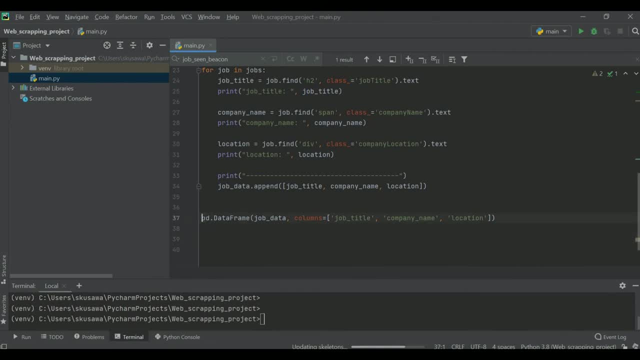 fine, our data frame is created and let me just name it like something df. uh, something df only can say like a data anything. and now if you want to print, you can just print this data frame dot head and you can see that how it is saving the all records. so let me just quickly run and show you. 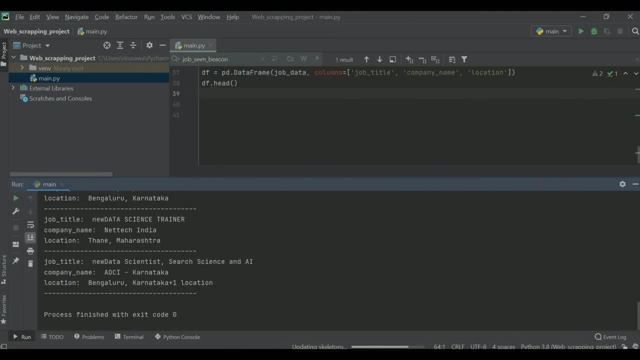 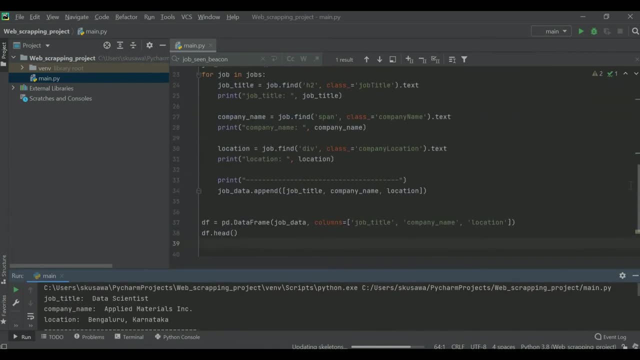 now our data would be in a tabular form. okay, so we are printing data. why it is not printed, okay? okay, let me just check. something is messed up. let me just go back and stop this printing now, because we are directly going to print from the data frame itself. 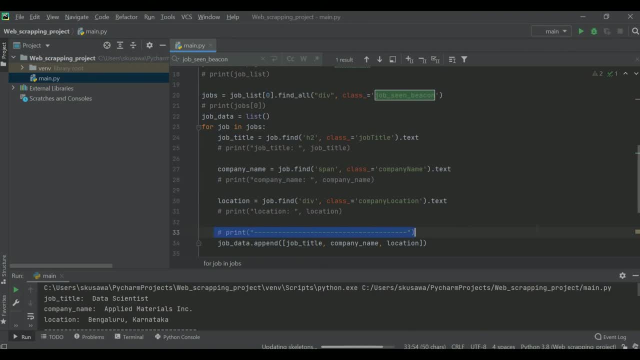 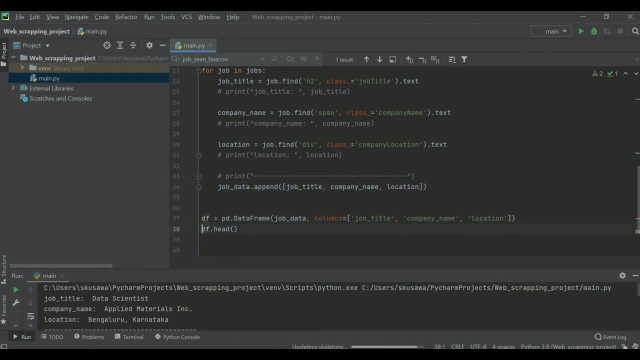 let's comment these lines- printing lines- and we are going to append each data inside of these. that is also looks good. okay, so i missed to print here. okay, so let me just print it and let's try. okay, let me just run now. okay, i commented all these lines which are printing the previous. 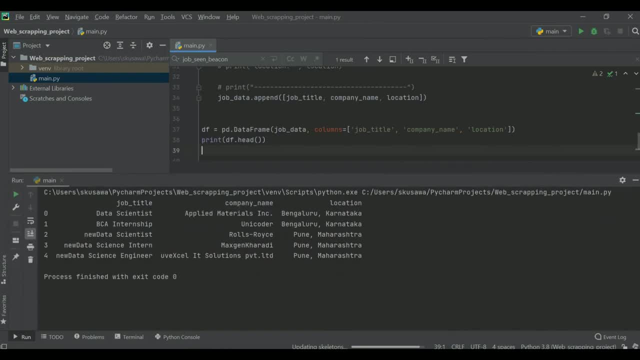 data. so now you can see that we have data in tabular format: job title, company name, location. i have just printed the five first row records so you can see this job title, company name and location. so this way you can prepare a data. if you quickly want to save this data inside of a csv file, then you all already must. 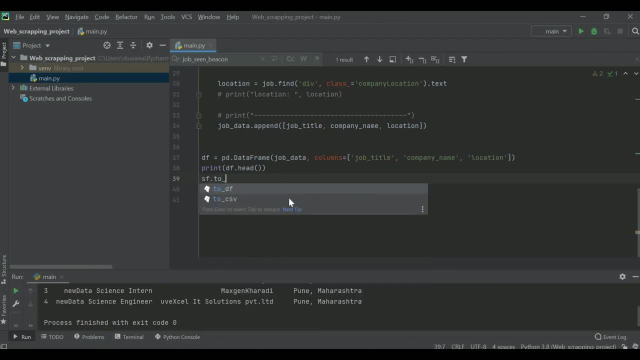 be knowing the data frame method, like data frame dot to csv, you can use and inside of that you can just pass your file name, whatever you want to give the file name, like any csv, like a data dot- sorry, data dot csv- and that's it. okay if you want to. 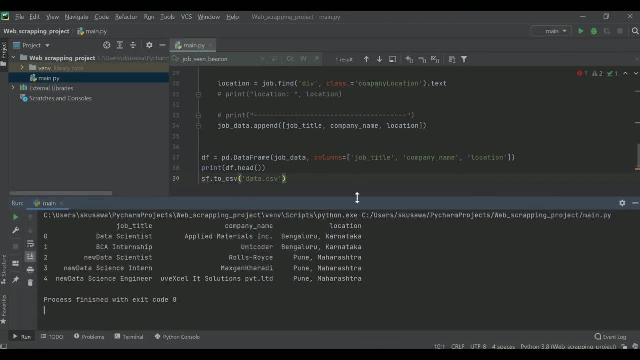 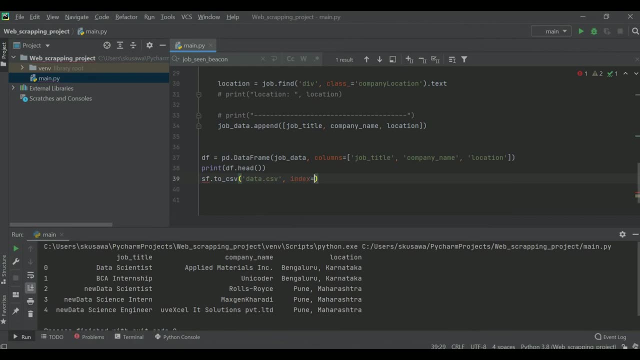 include these indexes. okay, then you can just keep as it is. if you want to remove these indexes, then you can just mention here: like index false, okay, so i just want to don't want to index include it, so i just say: like index, like false, that's it okay. data frame: okay. 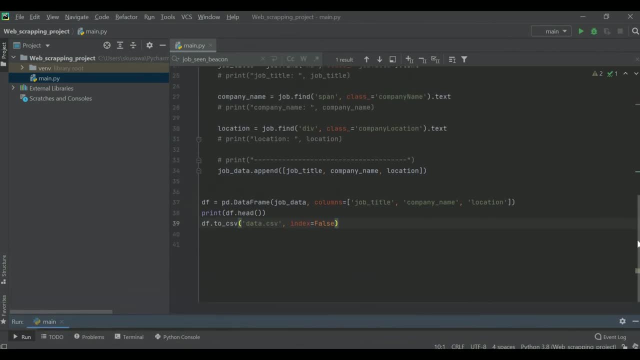 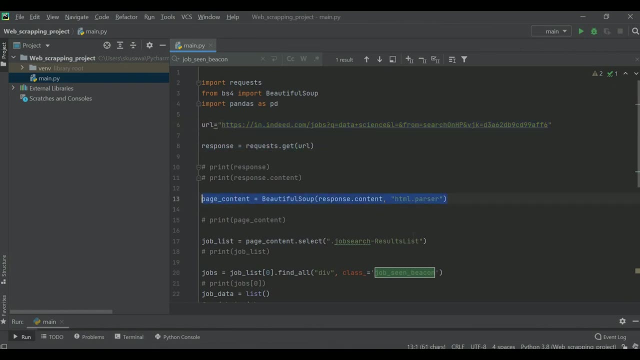 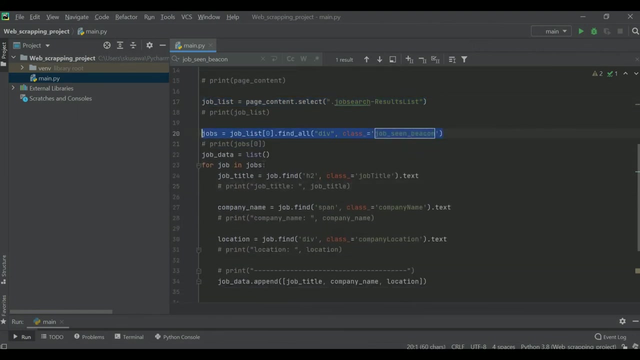 now we are just doing the web scrapping of a data. let me just quickly revise for you. we are just taking the url, we are fetching the data with a request url. we are parsing data with a beautiful soap in html format. we are facing the all job list and after that we are fetching the each job. and once we got the all jobs from, 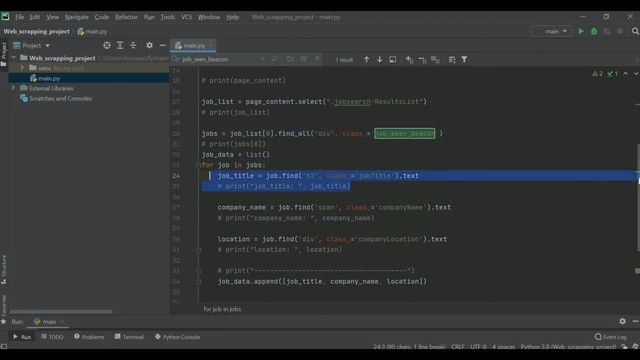 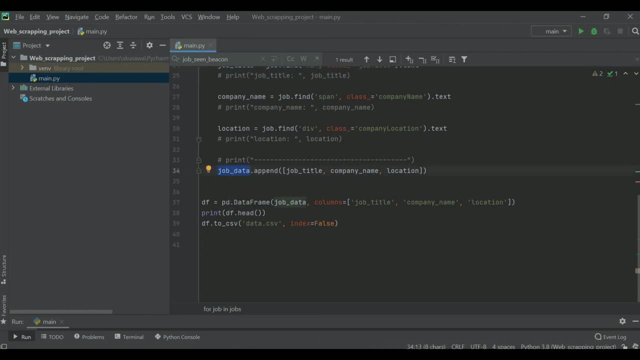 each job. we are trying to fetch the required fields like a job title, company name and location, and we have added into the one list and then from that list we have created a data frame so we'll get a tabular data form and then, if you want to persist or save that data, we are saving with a 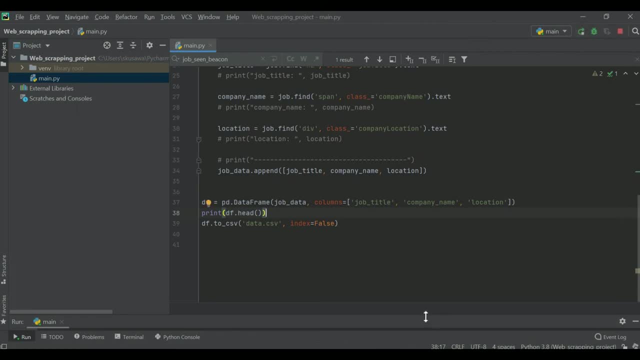 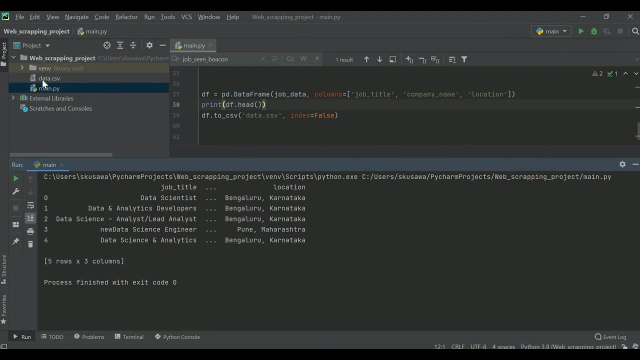 two csv. so let me just try to run and quickly show you. okay, so it is running. so let me check the logs. okay, so it is run successfully. and if you see here inside of my explorer, so this is the datacsv file created. if i just open it, so this is the file just we have created. so we have scrapped all this job. 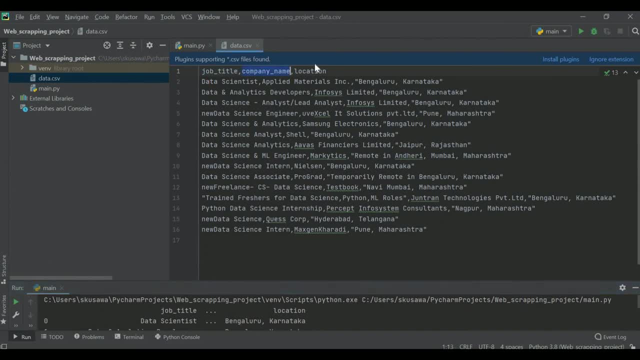 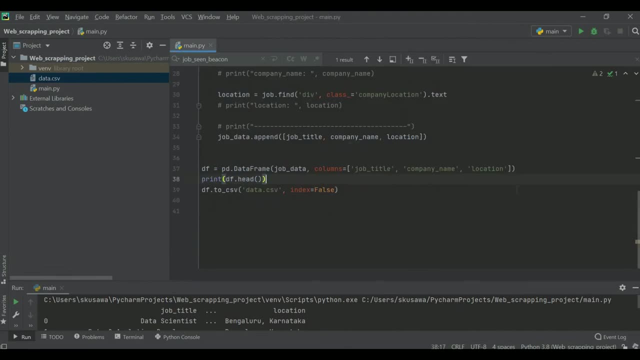 details, data from the internet with the three columns like job title, company name and location. so this way you can visit to the any page, access that page and, with the help of a soap ui, you will be able to access the different fields and extract data from that site. okay, so that's all about the